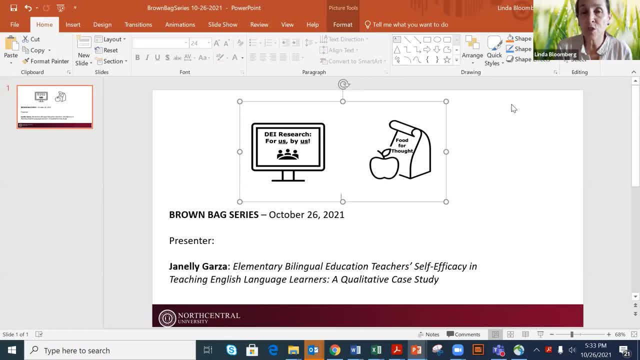 And the reason that I asked her to present is that not only does her research fall in the area of diversity, equity and inclusion, as you can see here by her title, Elementary Projects and Education, She's a bilingual education teacher's self-efficacy in teaching English language learners: a qualitative case study. 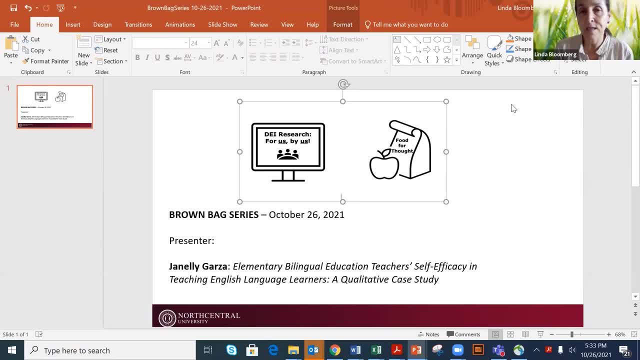 But Janelle has done such an outstanding- really outstanding- job of data analysis, so very thorough, that I really thought that a lot of other of the NCU community, both faculty students and alumni, can learn from her process, And it really is a great teachable moment here for us to learn from Janelle and she's going to walk us through her process. 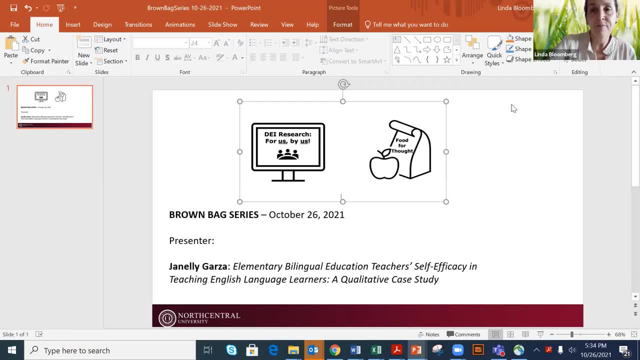 So grab your favorite Coffee, like I have mine over here. Grab your favorite snack. As we know, it's a Brown Bag presentation. It's informal. Janelle's got a great presentation for us. We'll give her about. I don't know however long. she needs about 20,, 15 or 20 minutes to present. 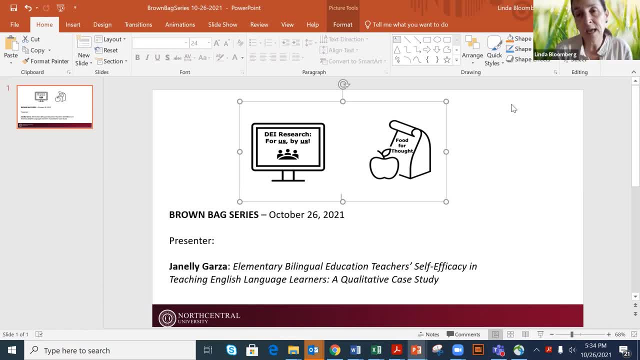 And then we're going to open up for questions And I'm really looking forward to the discussion and to you guys- everybody on the call- asking Janelle the questions that pop out at you as she talks about her analysis process with this very important study that she's conducting. 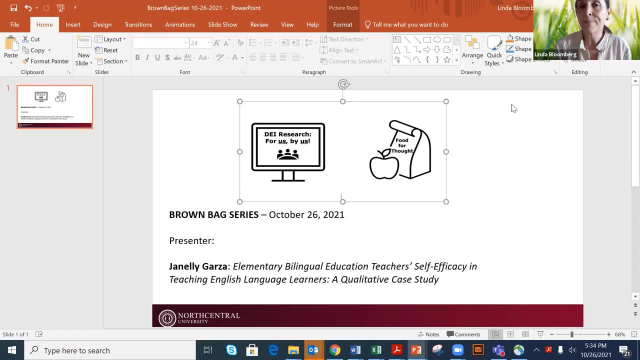 And, by the way, Janelle, she's almost complete, She's already writing up her findings and she's almost on her final dissertation chapter. So she's been a model student and I'm very, very happy. As you can see, she's really happy with her process too. 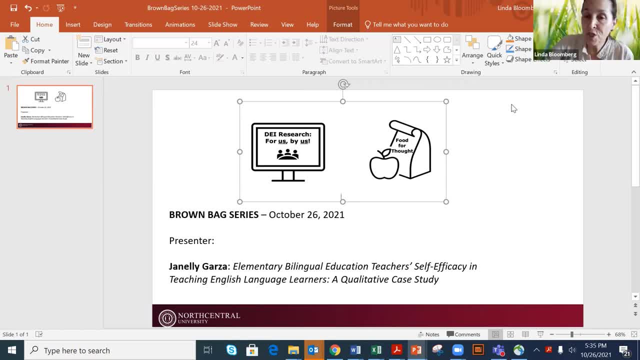 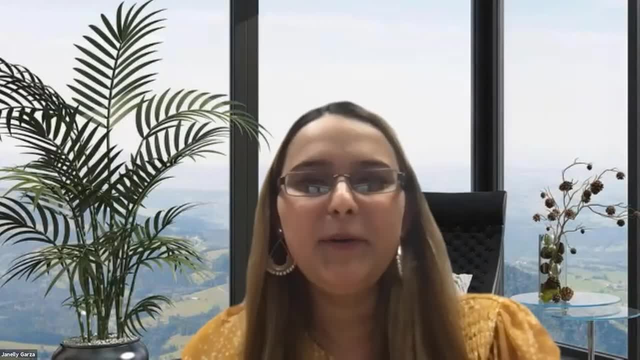 And so it's over to you. Janelle, Take it away, I'm going to stop sharing, And then can you please share your screen now? Yes, Thank you, Dr Pimberg, for everything and for your warm welcome. 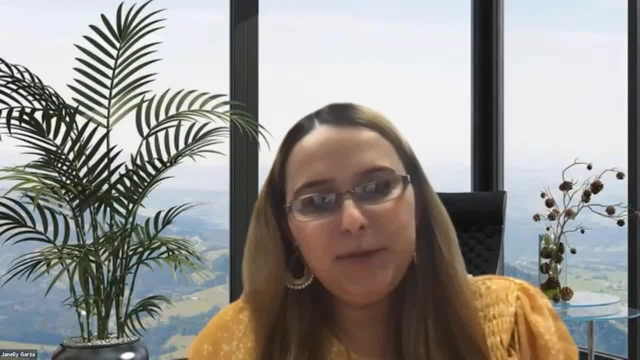 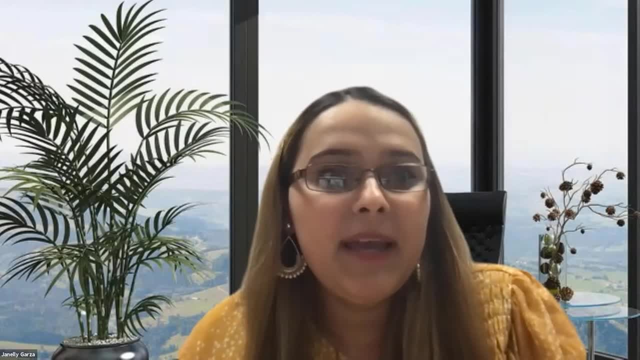 Welcome everybody. As I prepare myself to present, would you all mind stating on chat where you're from and where are you in the program, That way, in the meantime, I can start preparing to share, because I have many, many screens to share. 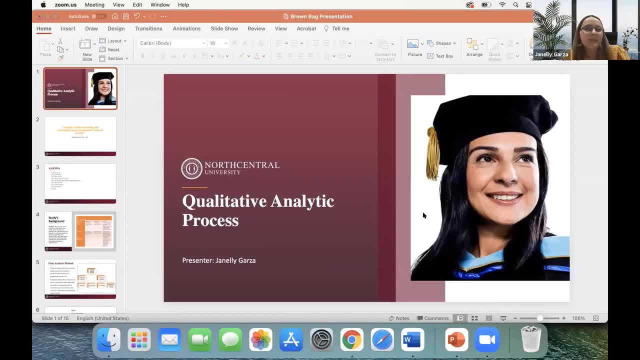 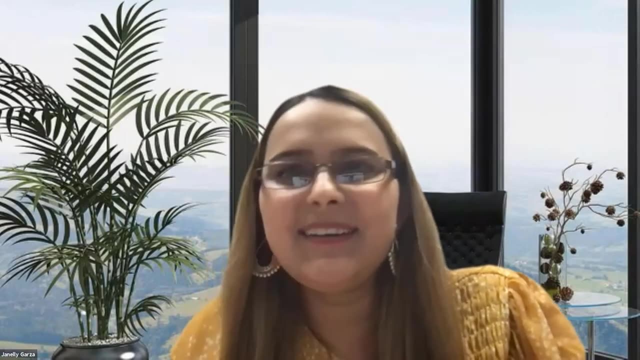 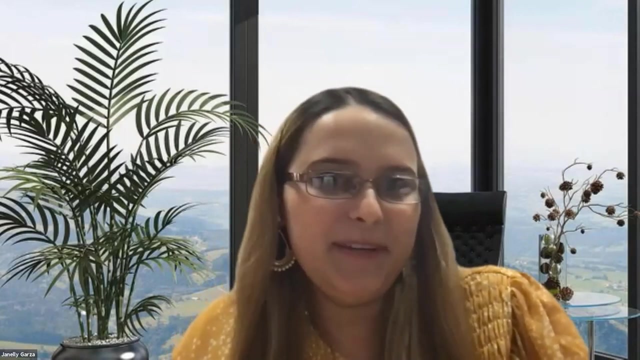 But, if you don't mind, just typing on chat where you're from and then where you're at in the program Kansas: Awesome, Welcome everybody. Thank you, Georgia. All right, well, it's nice to know a little bit about our people here. Phoenix. 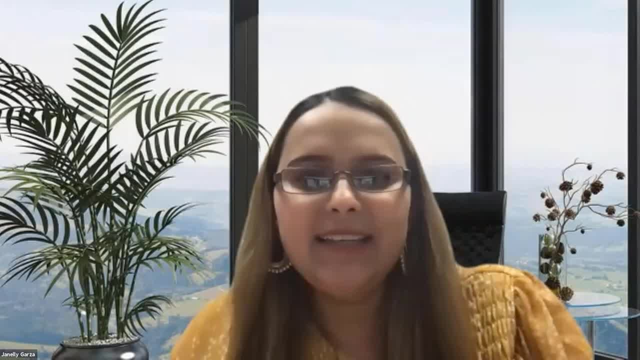 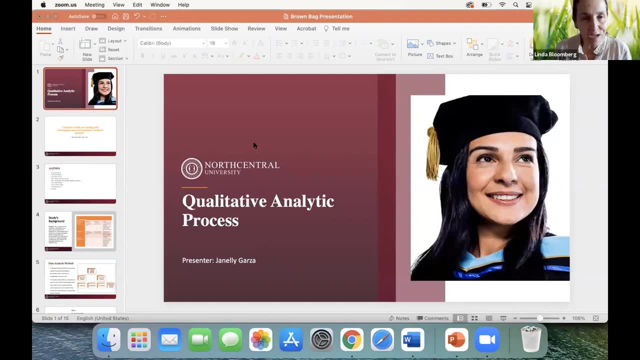 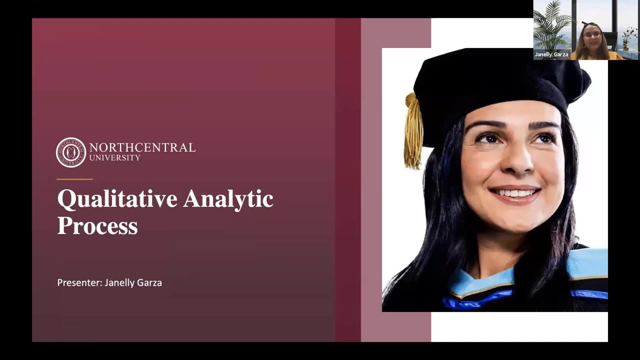 All right. So I'm from Texas and I'm ready. Here we go. Wow, you have a very big, very wide, diverse group of people from all over the country here. Janelle- Yes, I'm excited about that because, as you all know, I'm Janelle Garza. 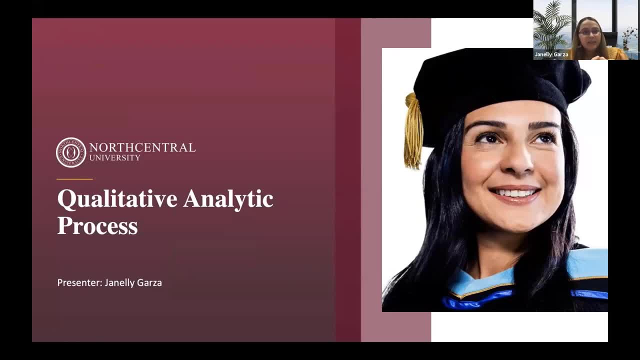 And I am very diverse- diverse. i'm actually hispanic, my parents are from mexico and i do live in the border with mexico, so i'm literally 10 minutes away from the border. i can commute every day if wanted to. so half of my life i was raised in texas and then the other half in mexico. so, yes, awesome, all right. so 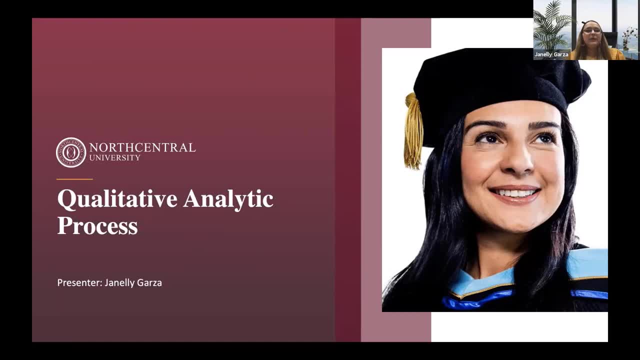 hello, i am miss janelle garza. today i will be presenting to you about sorry one thing. can everybody please switch off their put themselves on mute so there's no background noise for janelle. sorry to interrupt the janelle. i'm going to do so myself as well, no worries. thank you so much. 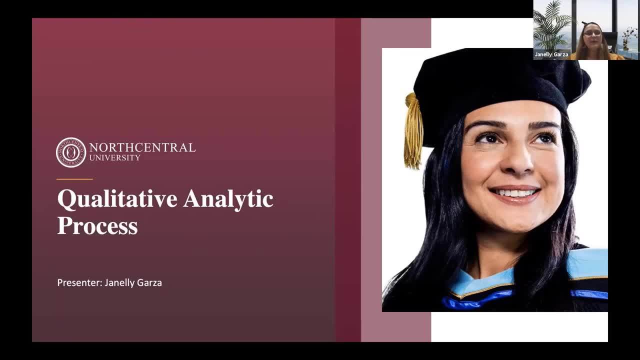 all right. so today i will be presenting to you about qualitative analytic process, and this subject is important, uh, because we get to see a broad view of how the analysis process looks like, um, in an actual dissertation. so i'm very excited, as dr bloomberg i'm about. 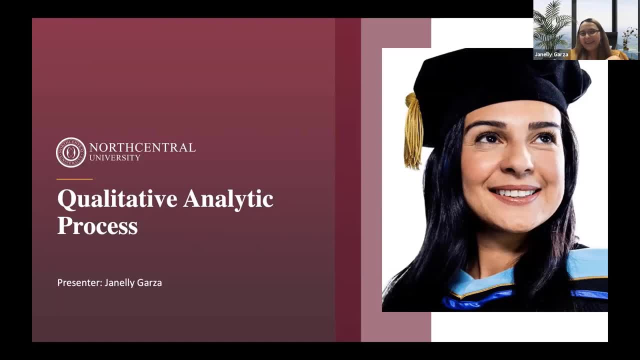 to be presenting to you about qualitative analytic process. so i'm very excited as dr bloomberg i'm about to be presenting to you about qualitative analytic process. so i'm very excited as dr bloomberg. i'm about to finalize section three of my dissertation and i can't wait. all right, 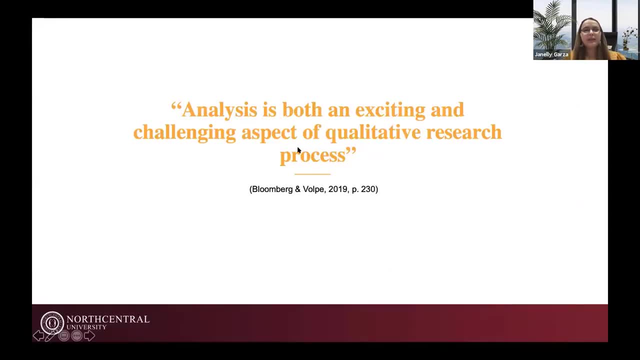 and then dr bloomberg, if you wouldn't mind letting me know, uh, five minutes before our time is up. all right, thank you, all right. so here is this quote that i wanted to start with. it says: analysis is both an exciting and challenging aspect of qualitative research process. 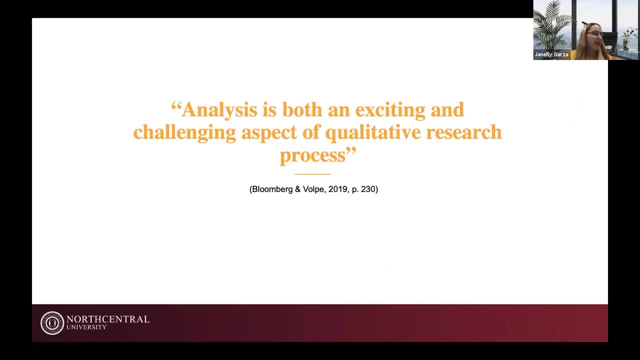 bloomberg and volk 2019, page 230, and actually this book, well, dr bloomberg's book qualitative dissertation: a roadmap from beginning to end, has been really, really my guide in my dissertation process because i followed it sentence by sentence, step by step, and i'm very thankful to dr bloomberg because 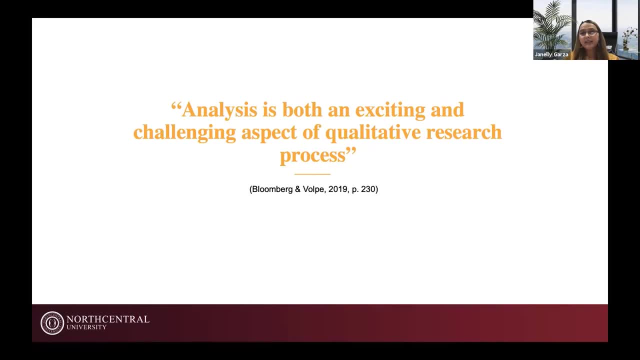 in stating this quote: um is, yes, exciting and challenging, and at moments when i really felt very overwhelmed- um- i'm going to share these words with you all from dr bloomberg- was that she told tina me that we only work on a dissertation once and for me to enjoy the process as i'm writing, and 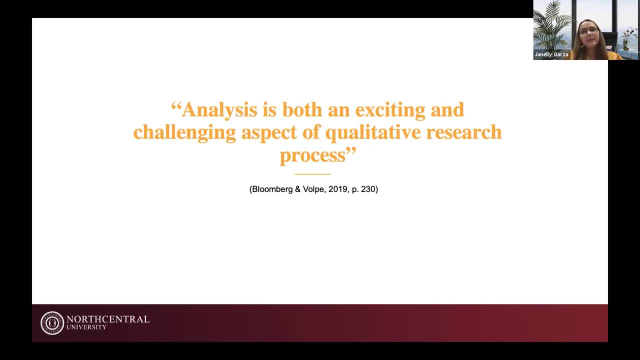 doing and spending time. so ever since that moment, my perception of having to sit down and write and do homework wasn't just sitting down, but my mind did shift and it was positively so. i did want to share that with you all. enjoy the process. yes, it's challenging, but it's also exciting because 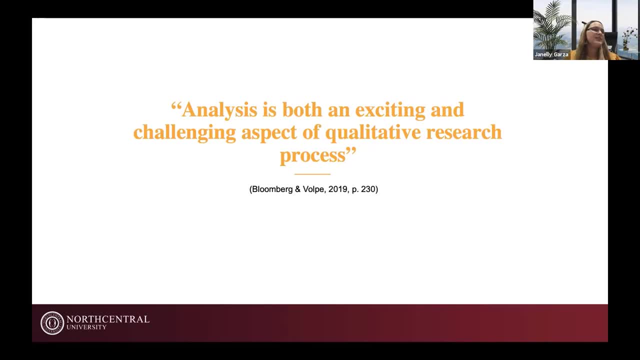 we only get to do it once and it's research and we're getting to get to see new findings. so thank you for that, dr bloomberg, and you're gonna hear me, um, quote her a lot, because all my study is based on her work. all right, so the agenda for today. i'm going to talk a little bit. 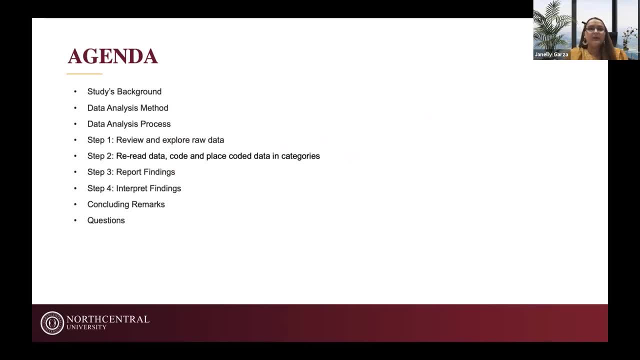 about my studies background: the data analysis method. i chose my data analysis process and i'm going to go through each step and show you all authentic samples of the data analysis process. and i'm going to go through each step and show you all authentic samples of the data analysis process. 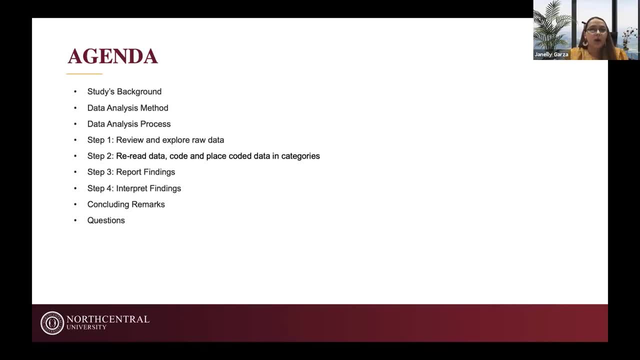 my work, that we all can have some examples and models um, that you can have an idea for. and then, uh, concluding remark, and we're gonna move it on into questions. so i recommend that you all have your little notepads, notebooks, so that, as i'm presenting, you can write your questions and we 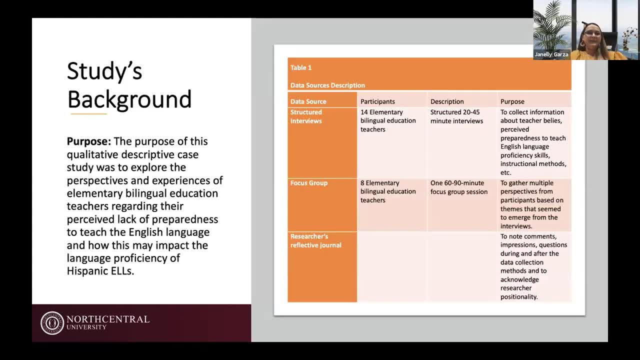 can have a discussion at the end. all right, so a little bit about my studies background. the purpose of this qualitative descriptive case study was to explore the purpose, perspectives and experiences of elementary bilingual education teachers and their perceived lack of preparedness to teach english language learners. we see here that i used structured 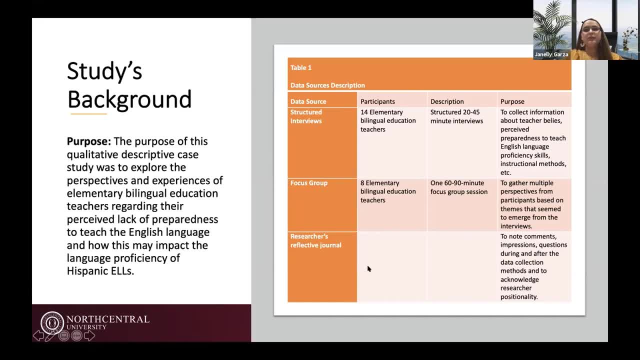 interviews, a focus group session and my researchers reflective journal. so you're gonna be seeing a little little snippets of each uh data component and then a description- they lasted 20 to 45 minutes- and then how long it lasted and the purpose of each. so this i actually gathered from my dissertation, section two. 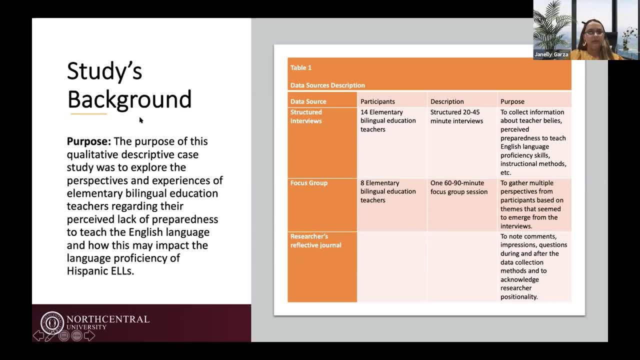 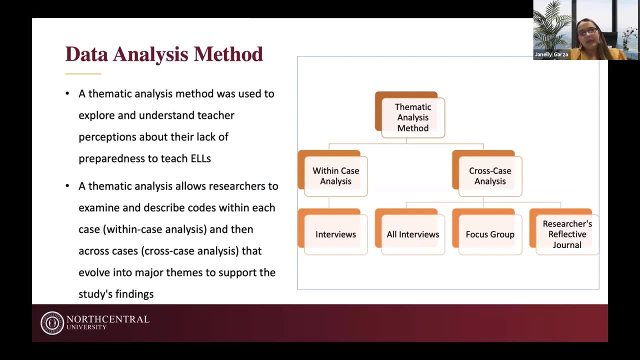 okay, so it's a little bit of my background. there we are. so my data analysis method: i decided to use a thematic analysis method to explore and understand the teacher perceptions about their lack of preparedness to teach english language learners. now, within thematic analysis method, we have within case analysis and cross case analysis. 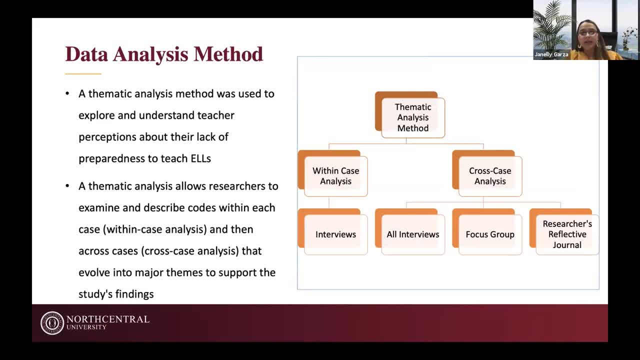 so a thematic analysis allows researchers to examine and describe codes within each case. so with i looked at interviews individually and identify, started identifying different codes as i went through the interviews and notice similarities and things that were present, and then across cases that evolved into major teams to support studies findings. 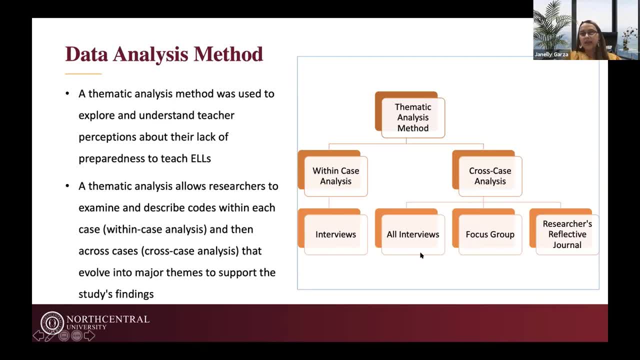 so then i started coding based on cross-case analysis when i looked at all the interviews and then included my focus on the interview sites and the Tallangal scores. now, when i looked at the interviews- focus groups session as well, And then my reflective journal, So I first used within case each interview individually. From there I went on and developed questions for my focus group so that I could code across cases. 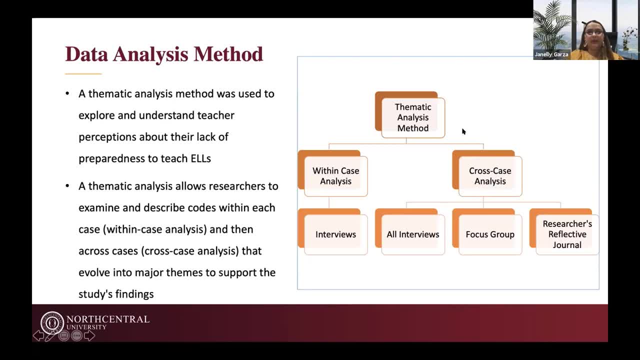 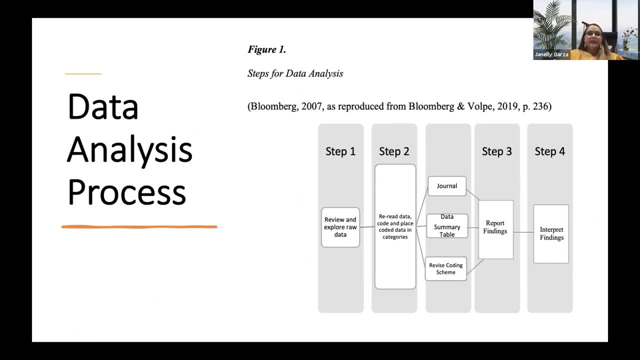 All right, All right. So the data analysis process. These are steps for data analysis that I borrowed from Dr Bloomberg and it is included in her book. I don't know if you can see this, but it's on page 236.. And I literally followed these steps step by step, guided by 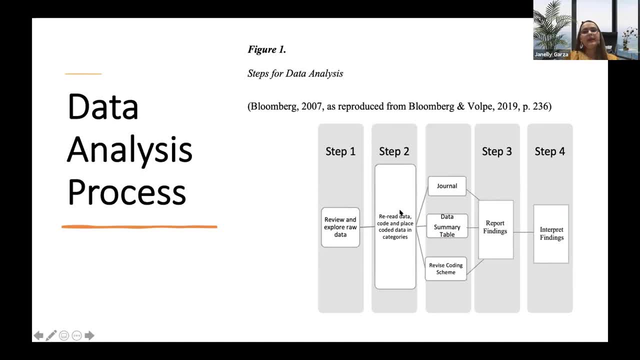 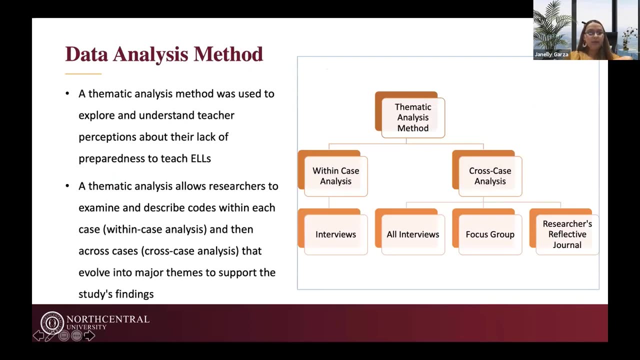 By the chapter, by what the book read. And so, step one, I reviewed and explored my raw data, which is when I did my- I don't know why, let me see- When I did my within case analysis through each interview. And then, step two, I reread the data, coded and placed codes into categories. 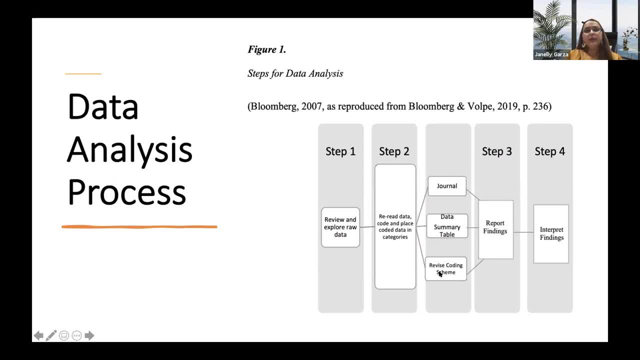 And here I included the journal data summary table, revised encoding scheme. So on step three. Step two is where we're going to see the major part of the coding and analysis process. Step three: reporting my findings. And then step four, interpret findings. And this is where I stand right now. step four, So almost there. 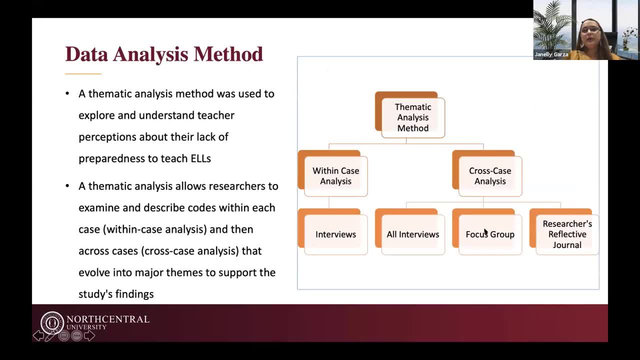 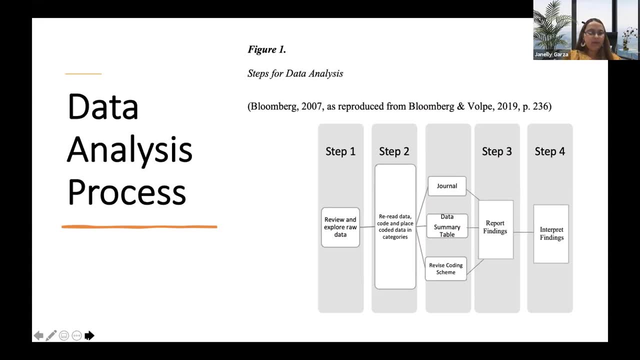 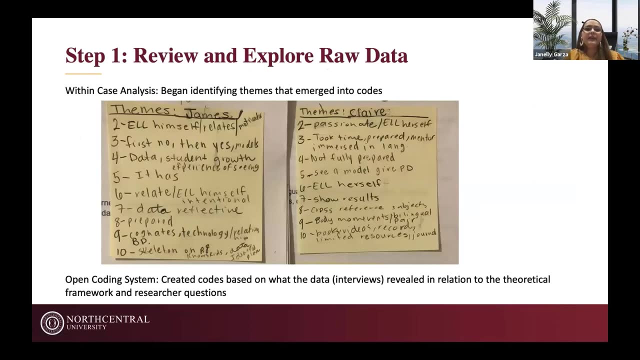 All right. And then just a quick example: that cross case analysis through the thematic analysis method was done in step two. Okay, So step one: review and explore raw data within case analysis. Again, I began identifying Themes that emerge into codes. So I individually looked at my 14 interviews and please excuse my handwriting, but I truly believe in providing authentic examples and models for others to be able to have. 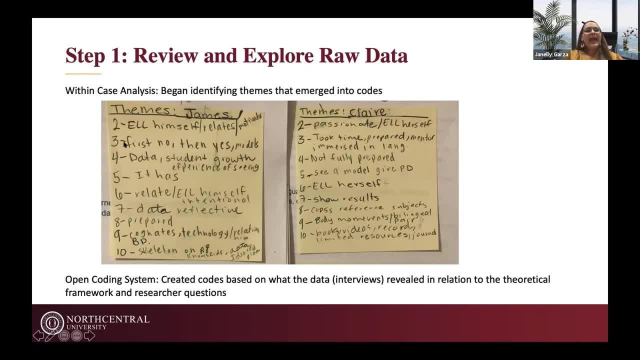 Right, So here's my authentic handwriting And I, as I was reading the interviews. I have different post-its. This is just one and I was writing notes. Okay, I see this. I see that these numbers here represent the questions on the. 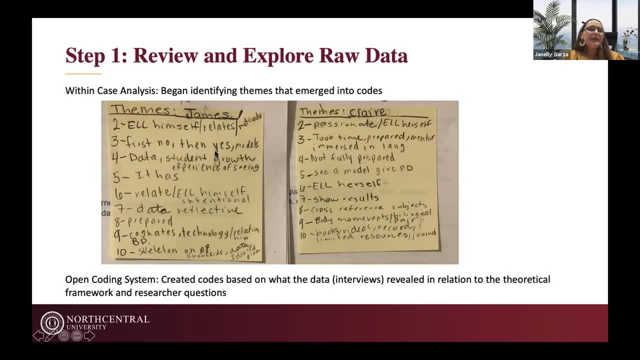 Interview guide. And then if you all are familiar with bachelor nation, you can tell them a fan, because my pseudonyms Came from bachelor bachelor characters, James and Claire. So for all those fans over there, So we see here, for example, number two, we see that James mentioned something about he was an English learner himself. 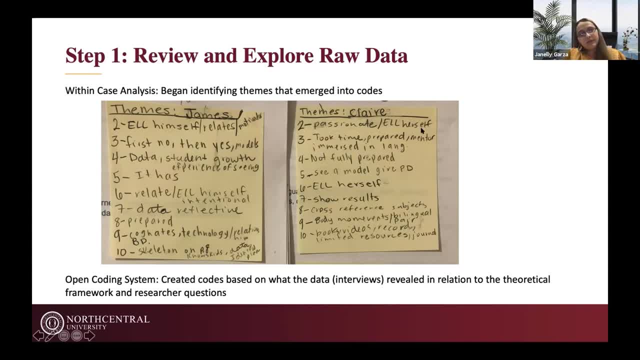 And then we see Claire mentioned that she was passionate and English learner herself as well. So guess what? So this is exactly The exact same thing. the exact same thing. Now I'm going to conscientiously click on that object here and see. 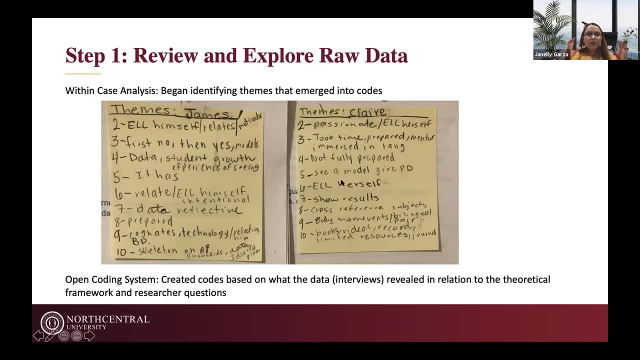 What we're seeing here. This is a lot of answers. One thing that I want to point out in here Is that Most of the participants, if not all, were English learners themselves, so that in Became an emerging theme. So there we see, and this is how I was making connection. 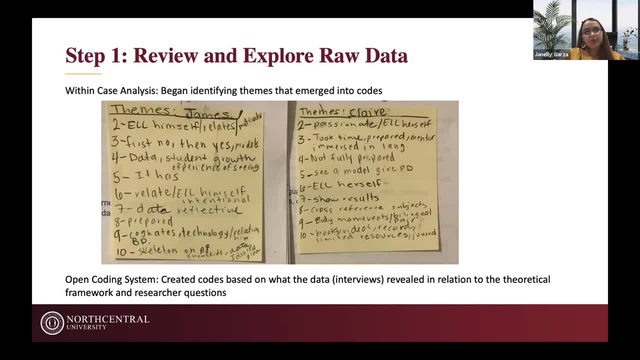 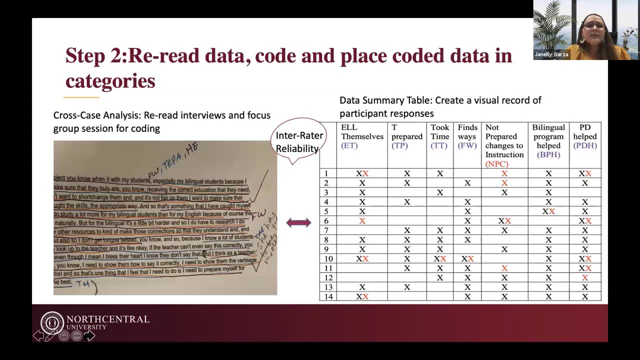 So it was a very big visual for me. theory and then bigotsky, social cultural theory. so yes, there we are for step one. step two: this is where i came in and re-read the data, code it and place coded data into categories. so a lot of. 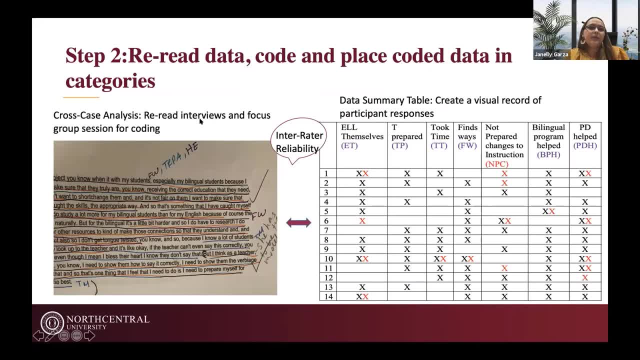 things happened here, so we see cross case analysis. i re-read the interviews and focus group session for coding. so remember, first i read all my interviews, develop some codes, develop my focus group questions based on what the interviews told me, and then i came back to my focus group. 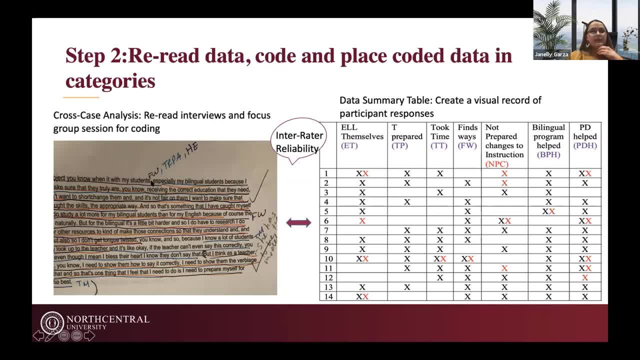 and my interviews to code, so see how this one sentence has different codes and i opted for a manual coding process where i printed out, made my notes. so this one sentence had all these three codes and you see different colored pens because i use different color prints to differentiate my 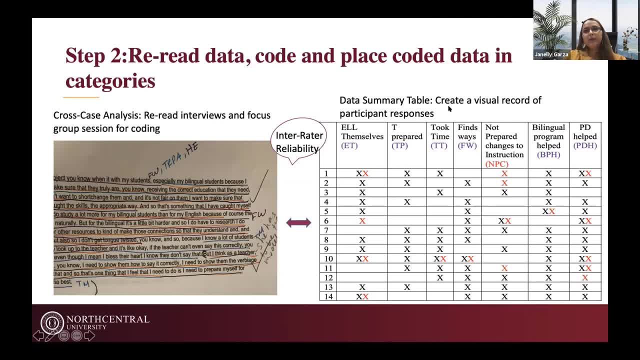 codes. and then we have the data summary table which, at the same time as i was coding, as i was also noting information on the data summary table which is also included in dr bloomberg's book- uh, very, very resourceful, um, and i had all my codes. 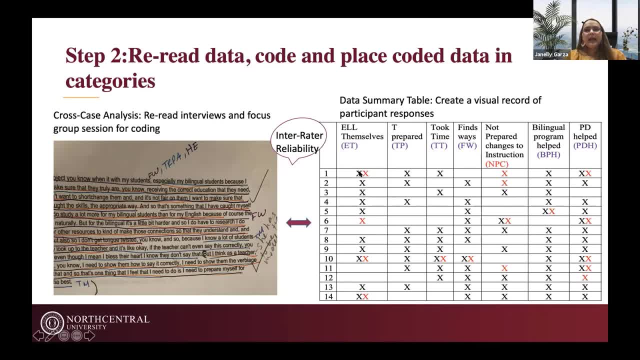 up here my participants and then i was able to represent okay participant. uh, one mentioned this that they were english learners in the interview. the red x's are the focus group, so this allowed me to even see my triangulation process across my data. so it was about it's about five pages long. 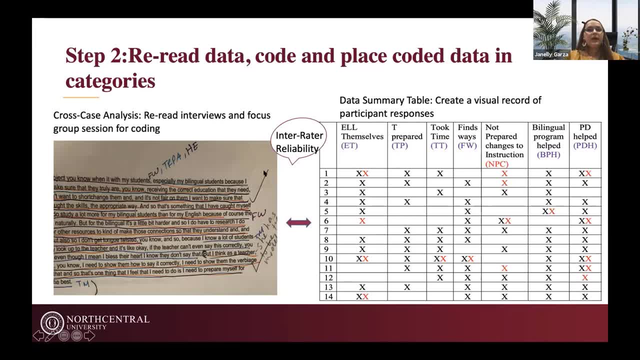 it needs editing, but it's a very, very awesome resource now. at the same time, while i was doing this, i also consulted with innovators- three innovators that are current doctoral students in the field of education- and they collaborated with me by coding some of my transcripts and i 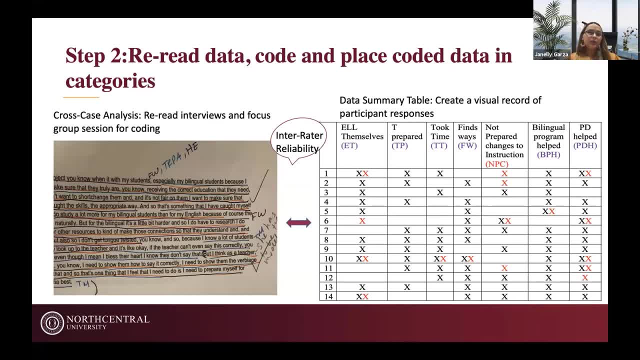 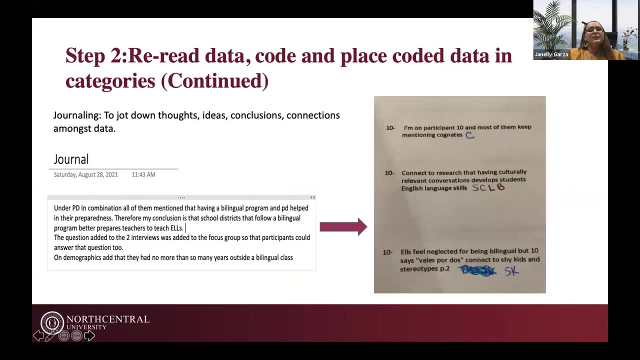 was able to compare what they found to what i had found and just question why i had quoted certain things, a specific way, why they had quoted other things. and yes, so let's go to the next step. step two: i again reread data, quote and place code of data into categories. 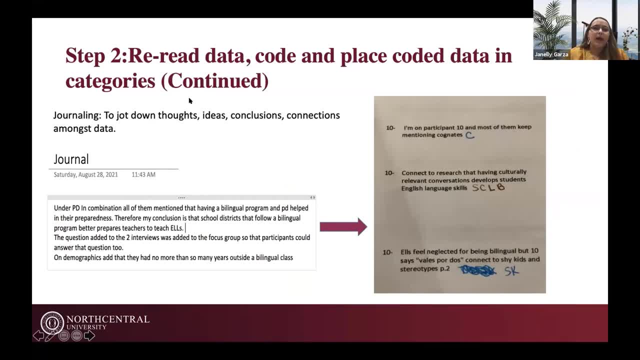 continued. so at the same time, while i was quoting and placing coding data into categories into my data summary table, i was also journaling. So I use Microsoft OneNote to journal, just because I type faster than I write. So this really helped me to make notes. And then I printed out my notes again because I'm more of a paper. 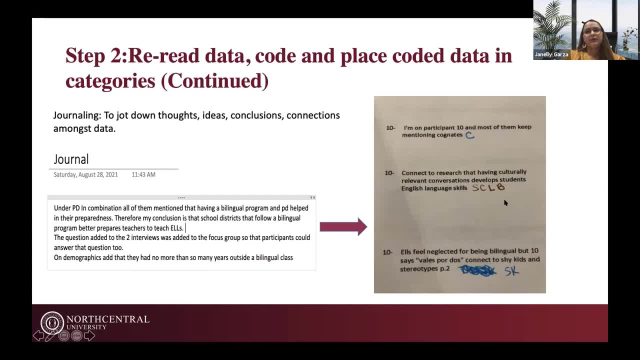 person And I went in and coded my journaling notes by sentence. So you can see here that C represented cognates, and then sociocultural, linguistic backgrounds, and then SK was shy kids. And here you see I edited because the code was teachers describing shy kids After talking to. 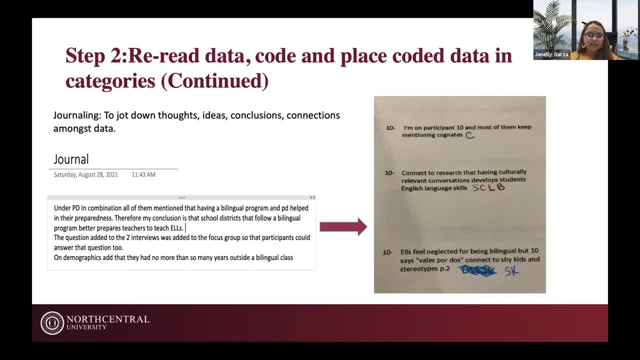 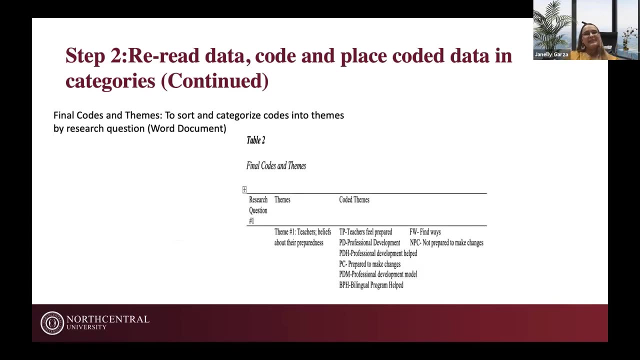 my innovators and collaborating. they say: you don't need such an extensive code. shy kids would just be fine. So this is an example of step two. All right, And continuing with step two, which is one of the longest process, At the end I brought my final. 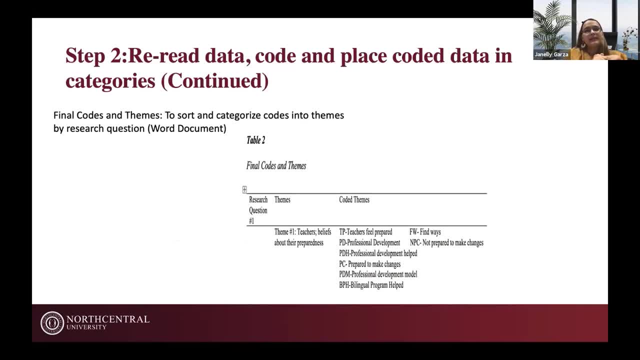 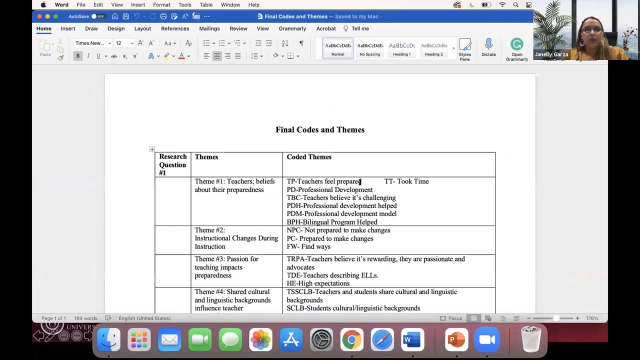 codes and themes And I sorted them out and categorized them into themes by research question. So here's an authentic example from my dissertation template- And I'm actually going to switch screens right now so I can show you a better example, which is here. So it's a Word document with my final codes and themes. So 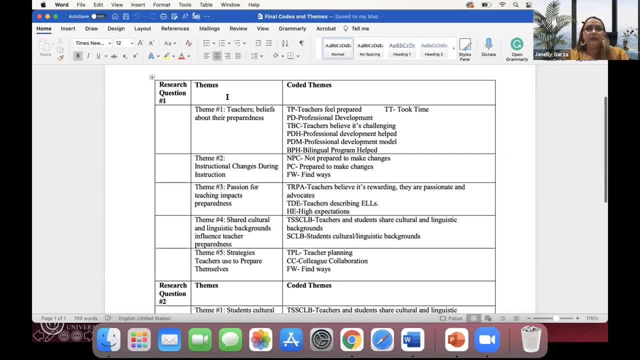 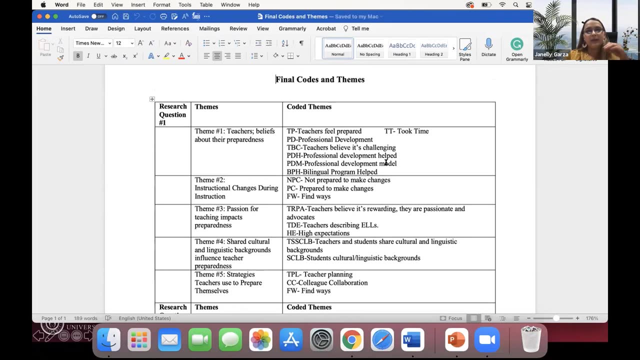 they're by research question. I was able to identify five themes for research question one And then the, the codes that fell under that theme, And this was very, extremely beneficial for me when I was writing my findings, because I would reference back to: oh okay, this specific code was targeted for teachers beliefs about their preparedness. 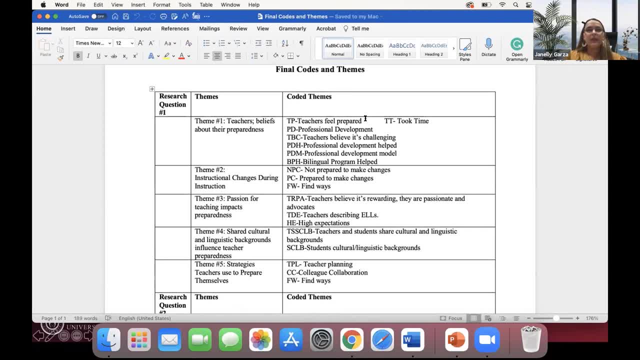 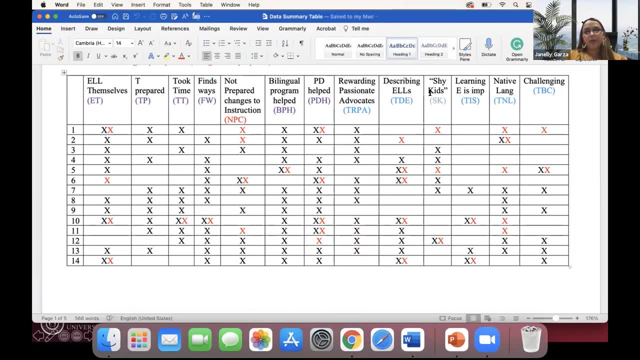 And it was just a lot easier for me to track. Now I would say, okay, teachers feel prepared, All right. so let me see in my data summary table which teacher said that they feel prepared, And, as you can see, it's a few pages long, And then I was able to go into those teachers. 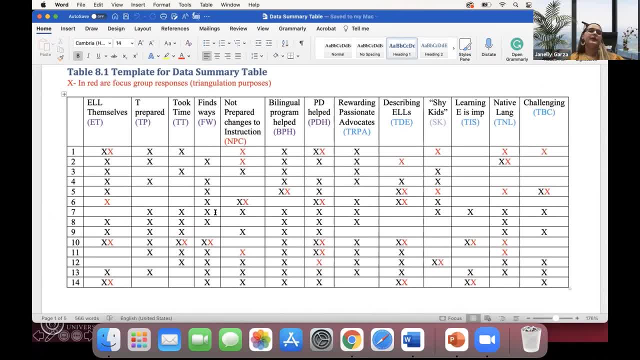 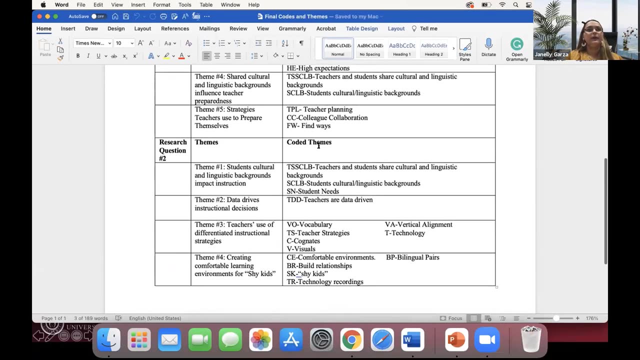 And look at my data. So it's a collaboration of bringing everything together, multitasking at the same time, but keeping everything for me organized by color in the files. Okay, and then we see research, question two by theme, and then my coded themes. I identified four themes based on my codes. 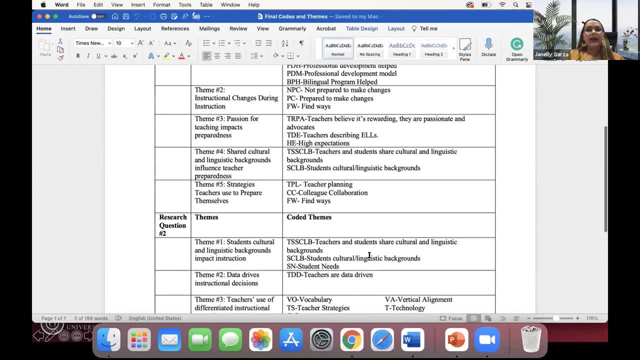 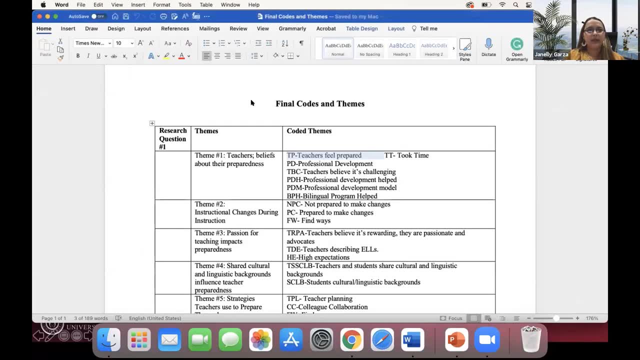 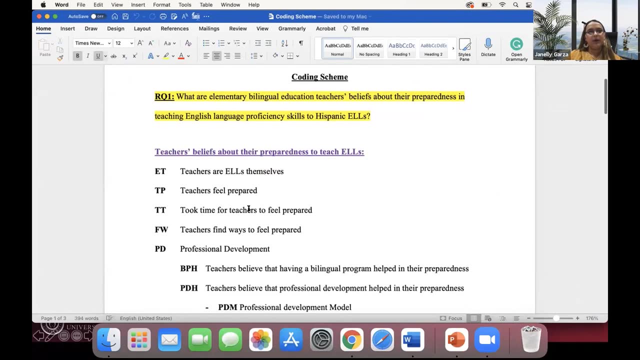 And there it is okay. And let me see, I have forgotten, wanting to get my coding scheme, my initial coding scheme. So here it is, my initial coding scheme, my themes And these were all the codes that I had identified. 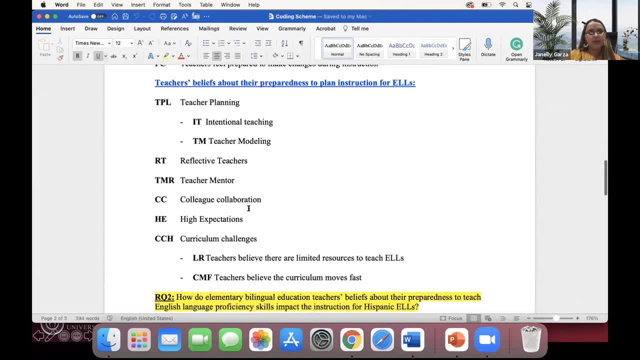 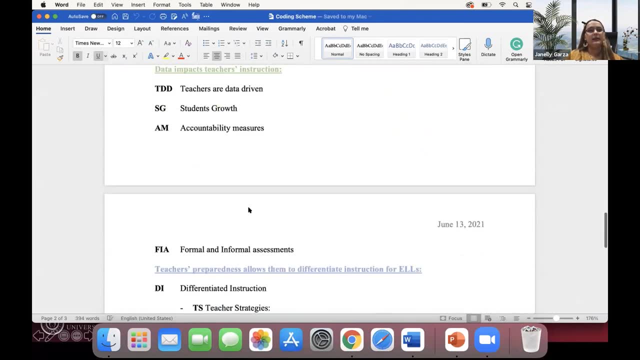 And then this I shared with my inner raters as well, so that they could have a reference for when they were coding. And it's again by research question, by color, And this is how they helped me. Now, all this happened in step two. 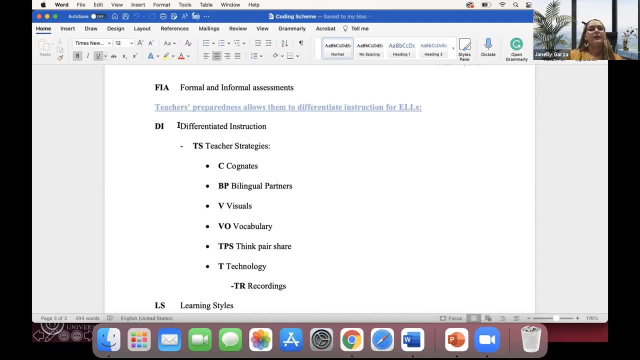 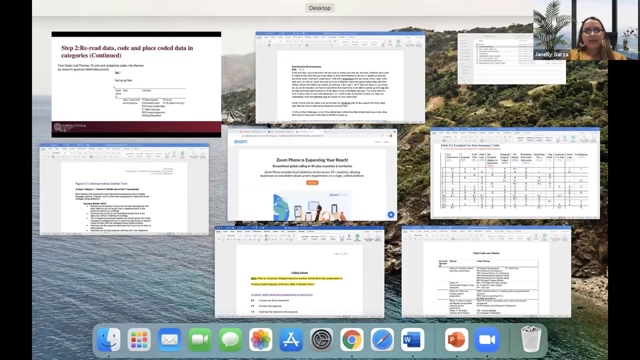 Now, as I print everything, I got the feedback from my inner raters And I went ahead and collapsed some of these codes. But I have it on paper. I haven't transferred it to this Word document just yet. All right, Now let me go back to my presentation. 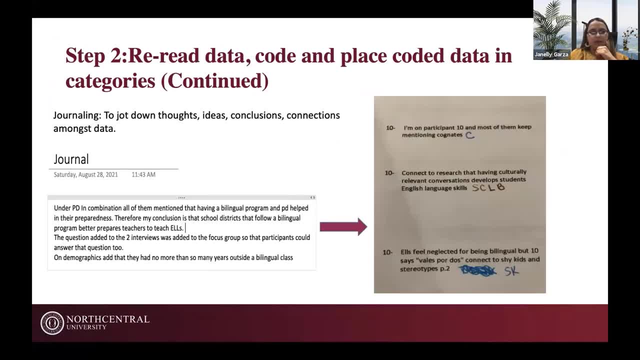 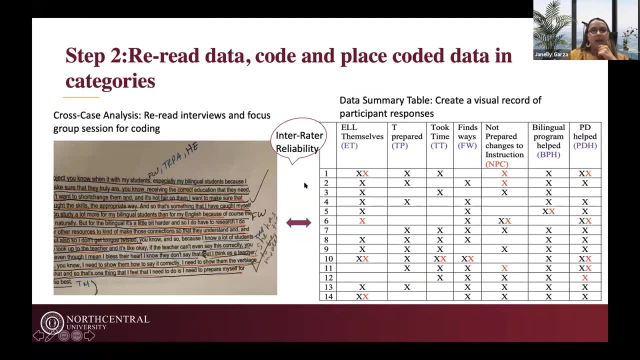 So we see that a lot of things happened in step two. I'm just going to give you a recap. So first I coded my data. As I was coding my data, I was jotting the data down on the data summary table. 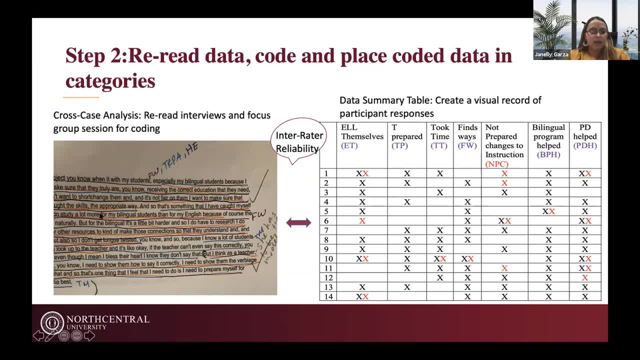 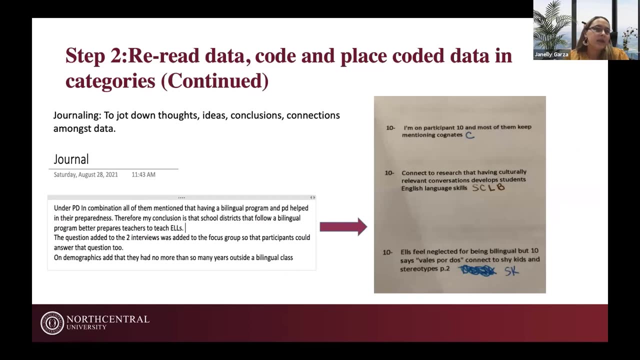 I did my inner rater reliability and compared my coding schemes to what other doctoral students had coded as well. At the same time, I was also journaling and reflecting on what I was writing, what connection I was making across participants, Any ideas that would just come up to my mind. 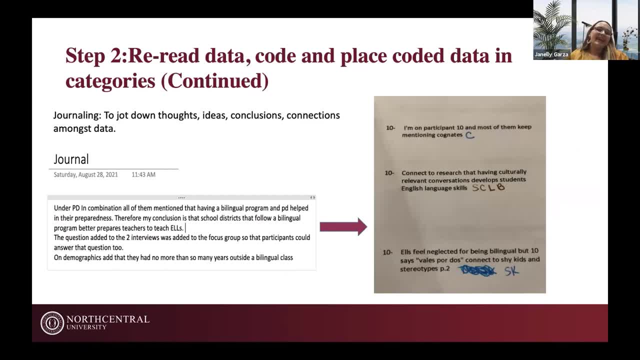 I would stop at that moment and write it, because you will forget. Well, I'm very forgetful. So I was like, OK, I need to stop and reflect this piece right now and why it connects to this other piece, and so on and so forth. 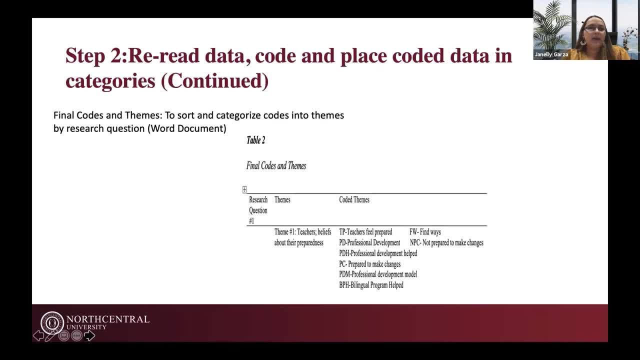 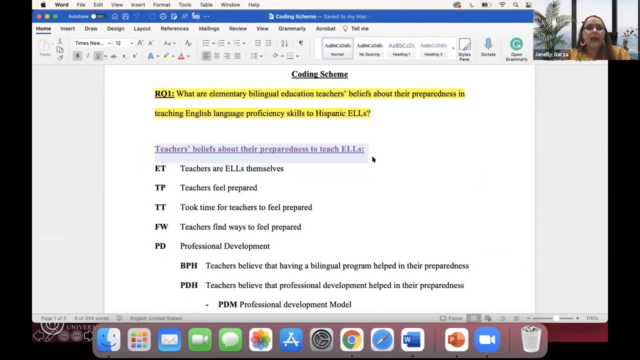 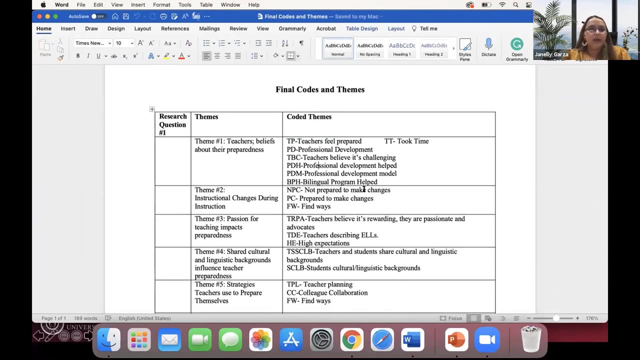 So that's again. this was at the end. I brought all my final codes together and based myself on my coding scheme. So from here is that I created these themes and then identified the coded themes that I wanted to use. All right, 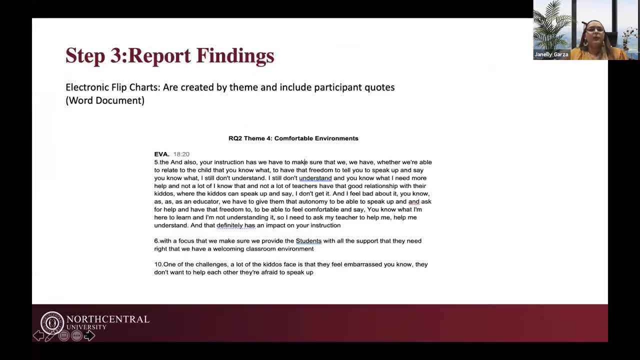 I'm going to go back to that, OK, So report findings. I've been using electronic flip charts, which are also included in the book, Very, very resourceful again, And they're created by theme and include participants' quotes. So this is an example that I used to create mine. 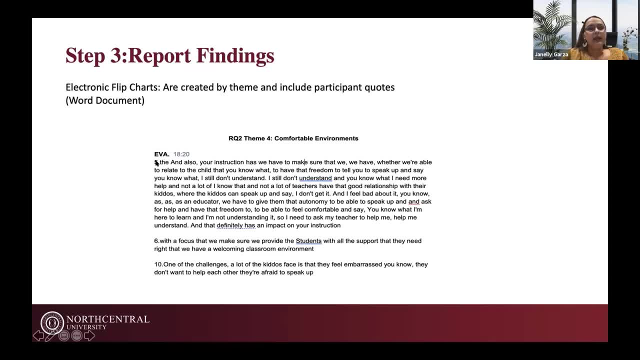 So here's another participant of mine, Eva, And then the numbers represent the page number that it has found, And I was just able to see all the quotes, So I just wanted to show you that. So here's another participant of mine, Eva. 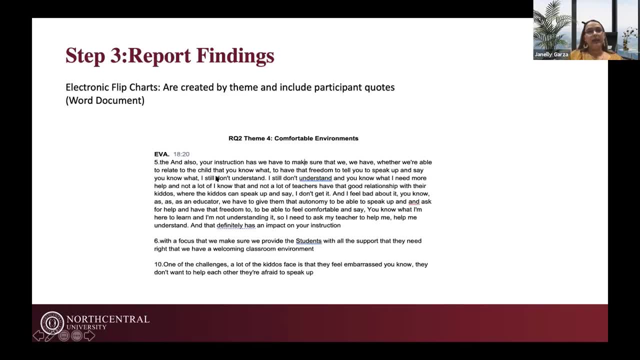 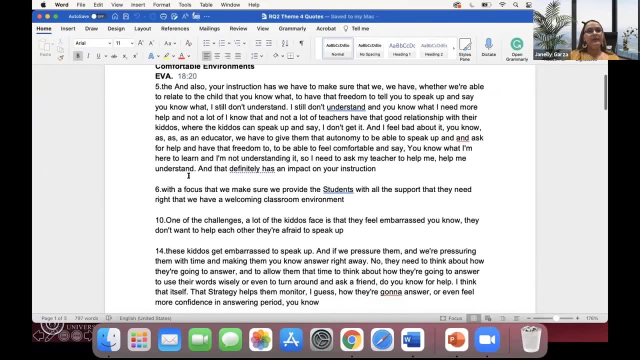 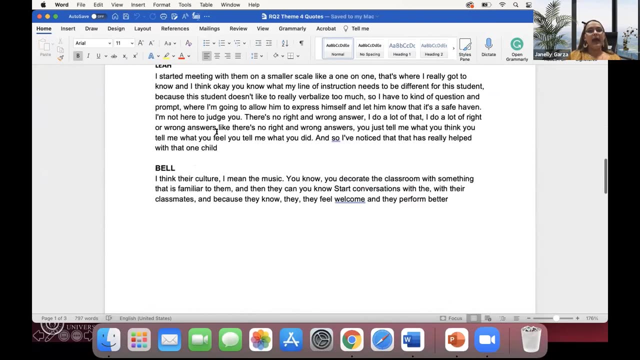 quotes that apply to comfortable environments and from there let me show you over here. from here I was able to see all the participants that talked about comfortable environments. I put all their quotes in the same page, again printed it, and this way I had a more visual of okay, which quotes. 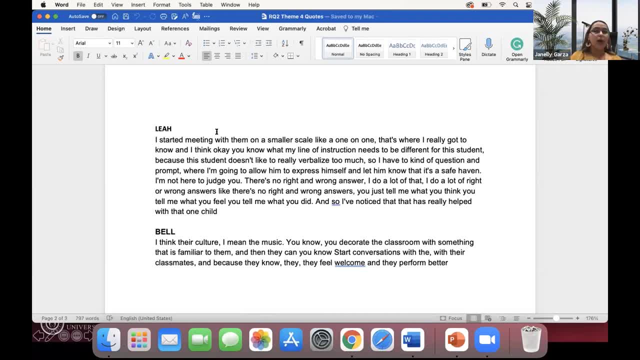 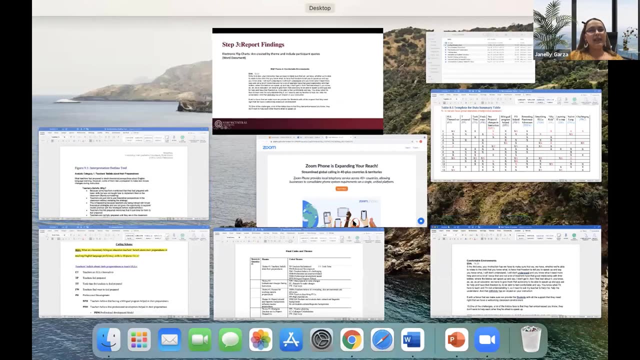 reflect a little bit more, the ones that that talk about my findings, which ones really target what I'm trying to say in my findings, to connect it directly to my findings. so this is how I did that and I just finished that step- if not last week, the previous week, but that's where we're at. 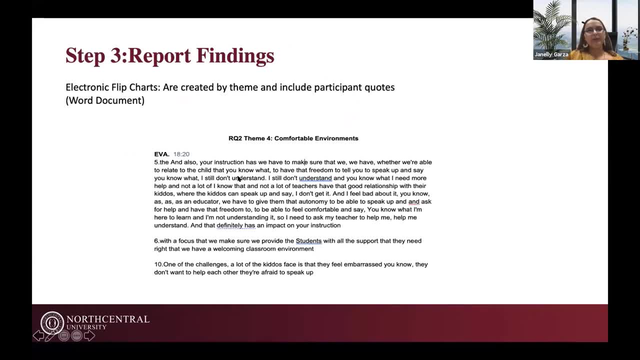 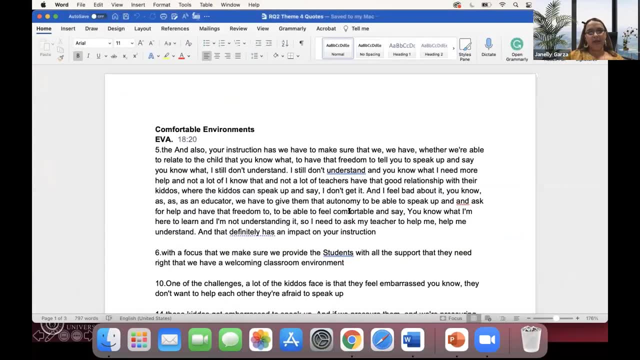 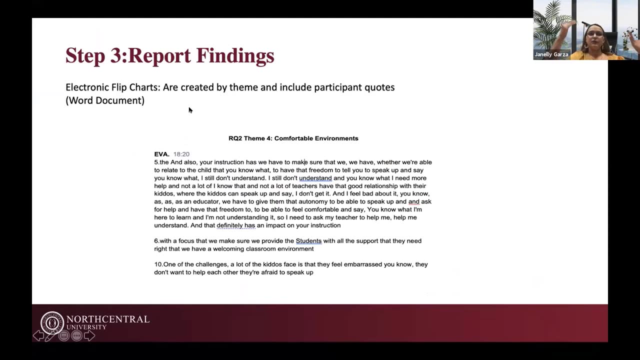 and it was really enjoyable. so for each theme here, we're gonna find one of these. okay, which is an electronic flip chart. now I know the book says that you could also do them on paper. you can cut tape the the quotes in a folder or so on, but this is just a way that I preferred to do it. okay, step four: interpret your. 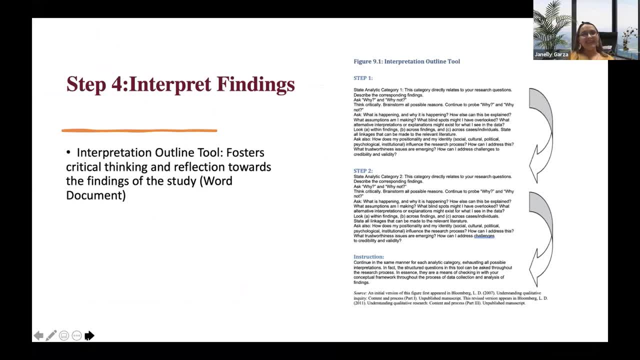 findings. so I'm using an interpretation outline tool, again from the book reference, and it fosters critical thinking and reflection towards the findings of the study. so it really, really got me thinking about why am I making this statement, why am I predicting that teachers beliefs are guided by their cultural 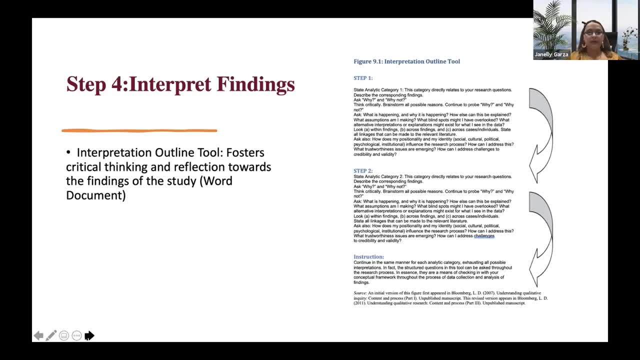 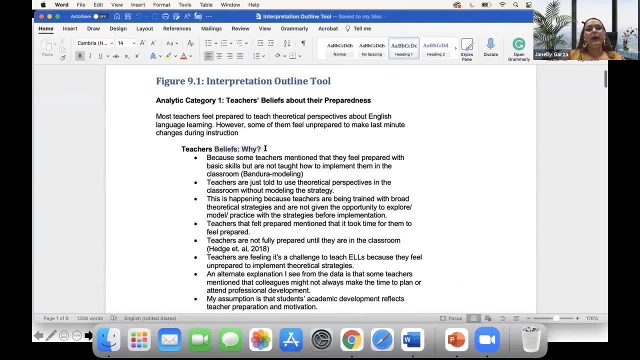 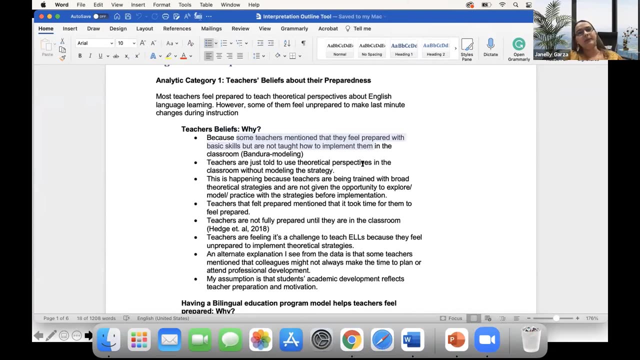 beliefs or so forth, or their short linguistic and cultural beliefs with students. so the interpretation outline tool really got me thinking about why and asking myself: okay, so why? because some teachers mentioned that they feel prepared with basic skills but are not taught how to implement them in the classroom and see how he or she can implement them in the classroom. 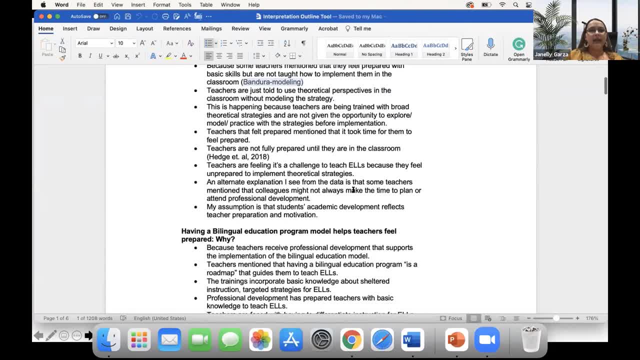 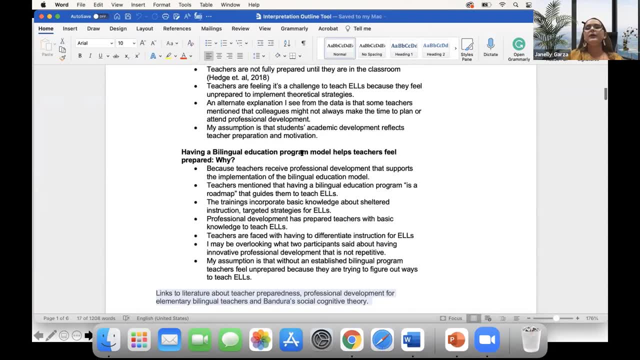 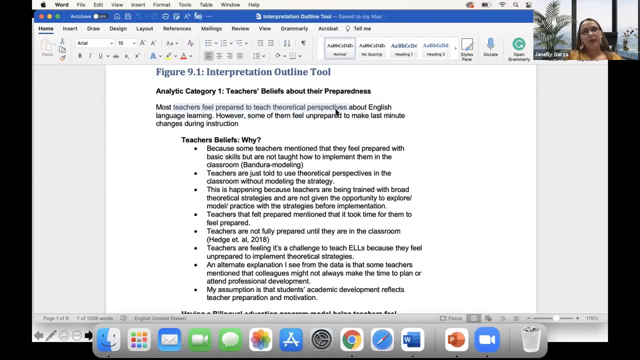 here I even connected it to my theory and then having a bilingual education program- this is another theme- helps, and then how it links to theory. so it's just really questioning reasoning why teachers feel prepared to teach a vertical perspective. so at the end my findings were that 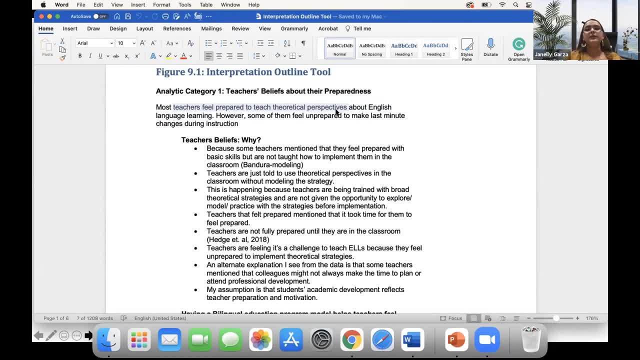 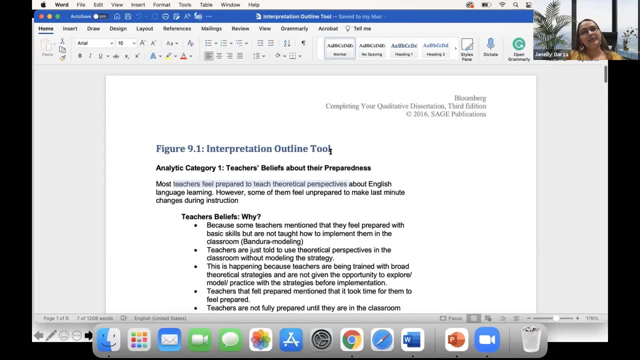 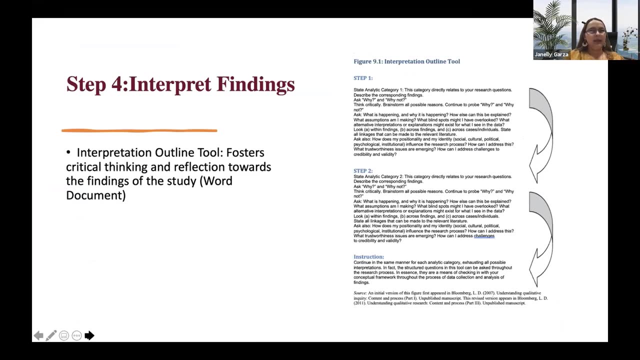 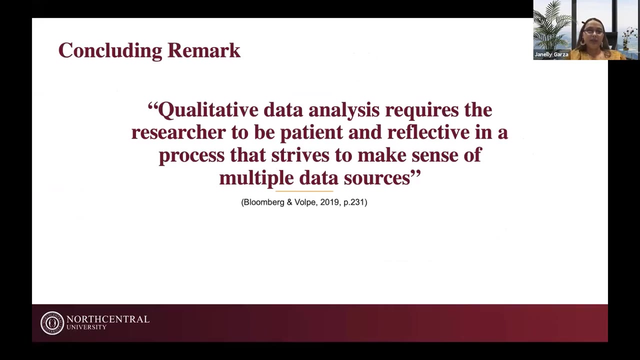 teachers Hispanic in elementary bilingual education. teachers do feel prepared to teach English language learners here in South Texas, and I specify the reasonings behind it. okay, so that's how the interpretation outline tool looks, and then my concluding remark is that qualitative data, data analysis, requires the researcher to be patient and reflective in 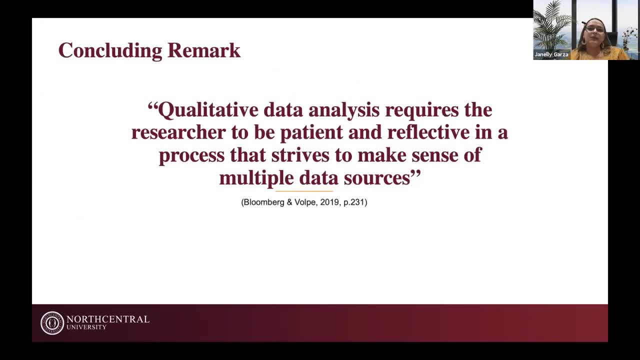 a process that strives to make sense of multiple data sources. so, as I mentioned earlier, um doctors, Dr Bloomberg's um saying, in which we only do this once for us to really enjoy it. and it does require us to be very patient because a lot of things are not in our hand, but it's up to us to. 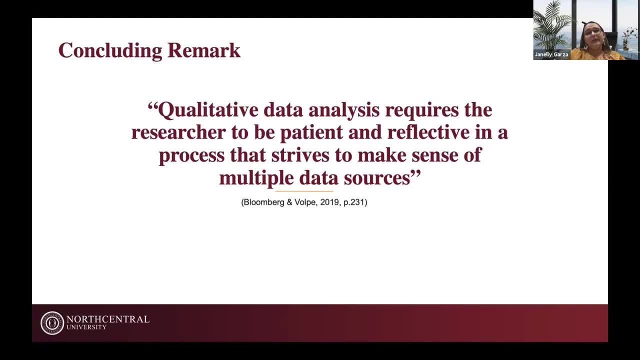 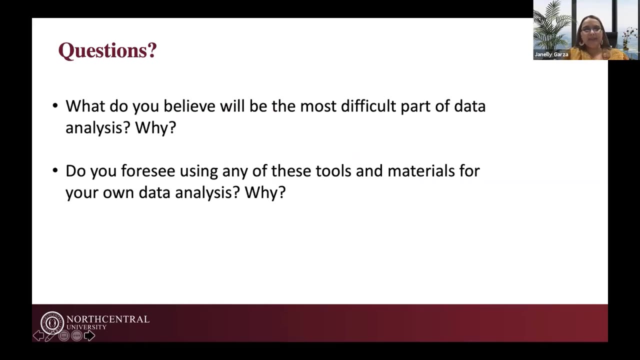 really focus and read and be patient in the process and, at the same time, enjoy it. um so, yes, because we're trying to make sense of a lot of data sources, all right. so right now, before we actually conclude, I do have a few questions for you on what would you believe will be the most difficult part. 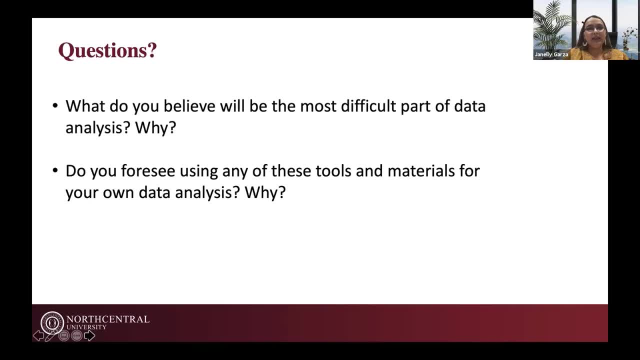 of data analysis and why do you foresee using any of these tools and materials for your own data analysis, and if you could specify why so at this moment, I would allow you all to ask any questions. that was an outstanding presentation generally, thank you. I'm so proud of you and all your work. 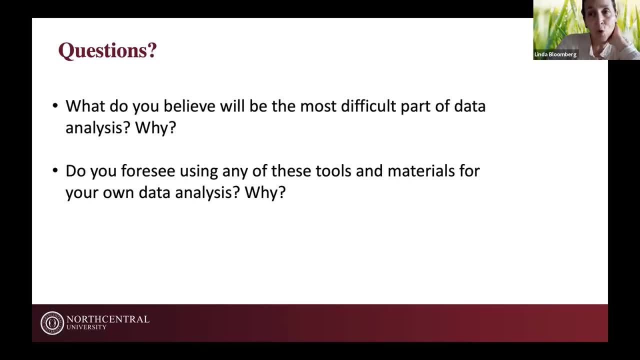 and your hard work, um, and these are great questions, so please all feel free to unmute and ask generally these, answer these questions and ask for any other questions you have about your data analysis process and anything that's on your mind now. she's given you a lot of information. 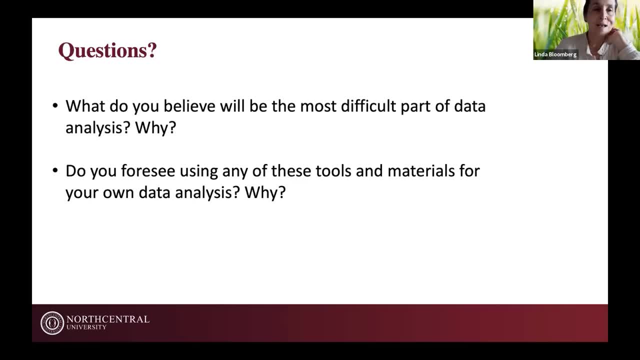 and um, what a great study. I have to say thank you. it has taken a lot of dedication and reading and, more than anything, being patient with with the process itself. yes, yeah, yes, now you all, don't be shy. and while everybody's getting ready to ask you questions, because I think they're all thinking a lot of oh, 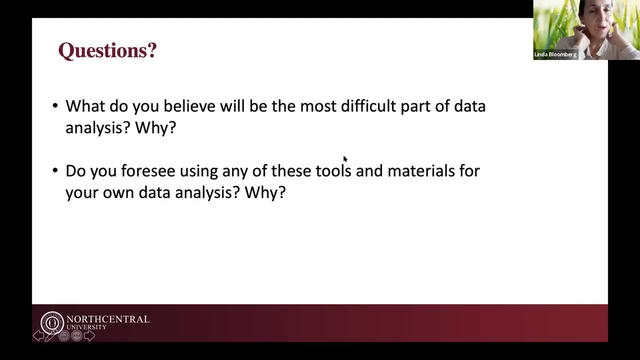 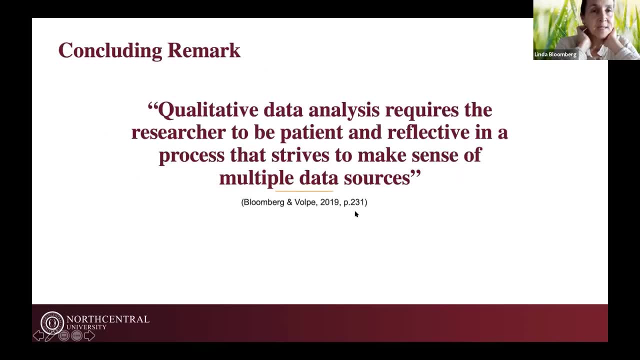 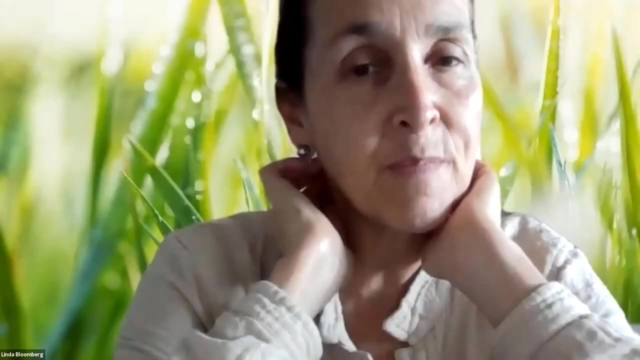 there's: um, I don't know if you want to say anything normal. I see your- your wonderful comment about an outstanding presentation. um, I just want to say that janelli really took her analysis, as she did with all aspects of the study. she really took the analysis to heart in a very, very methodical way. 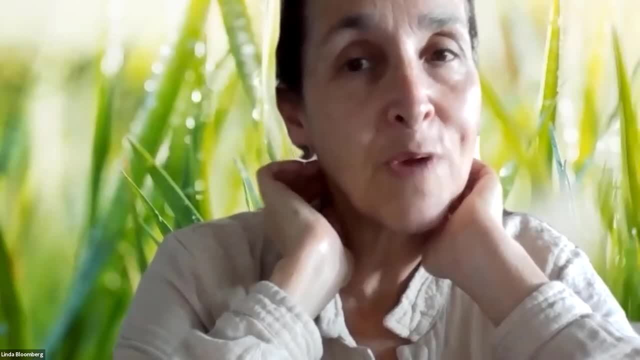 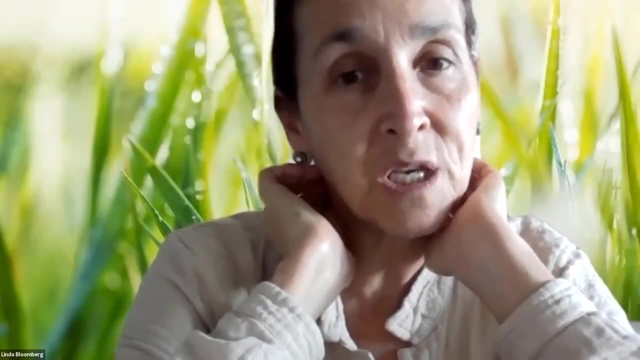 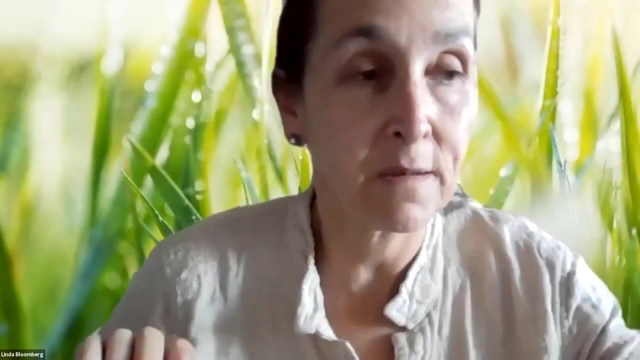 and she really was very, very focused on doing it correctly and comprehensively. I think it if writing saying: Janelle, you set for yourself a standard that you wanted to achieve and you didn't want to just do um a half-hearted job on this. you really wanted to do it um excellently. 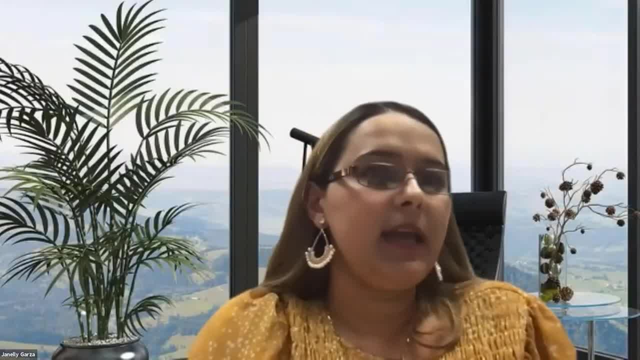 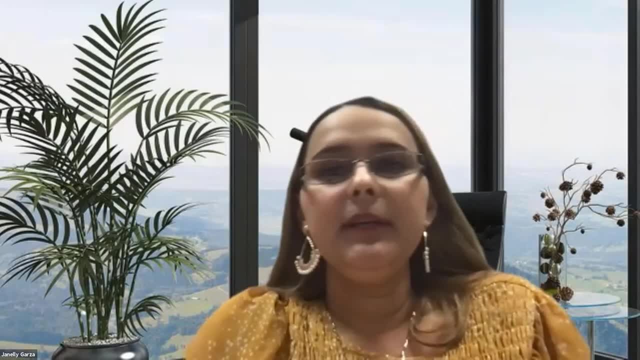 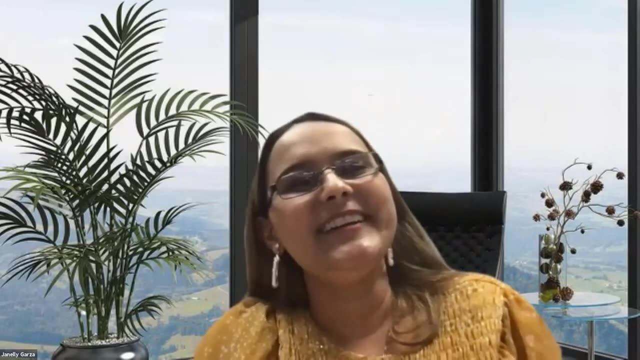 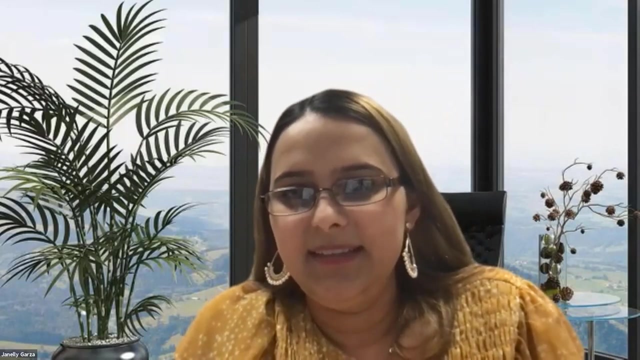 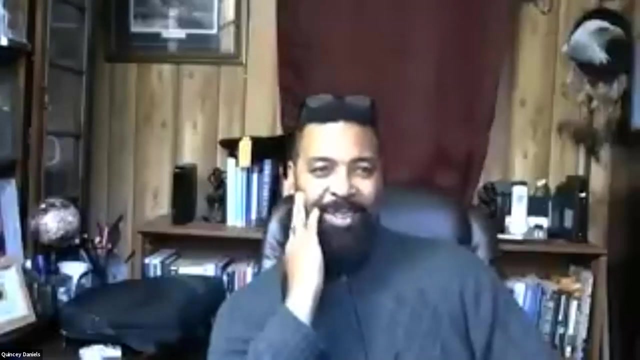 yes, and even to this day, on step four, um, the evaluation of the findings, of the outcomes, really looking into the literature connecting to what others have said about my findings and making sure that they specifically target my findings. so what questions? oh, go ahead, sorry, Quincy. go ahead, Dr Daniels. oh, oh, no problem, I always have. 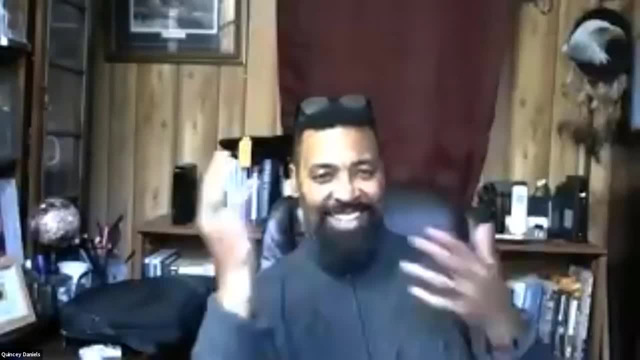 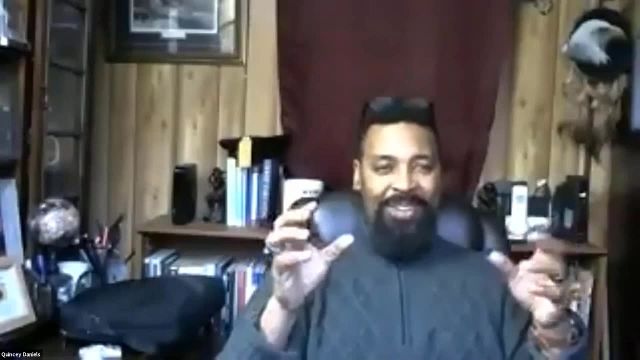 this idea. it's like when you're getting all the data- how in the world- because I'll have this with a lot of my students as well- when you're trying to figure out your codes and your themes. it's like I always had that picture of a beautiful mind where everybody's taking a string and they're trying to connect. 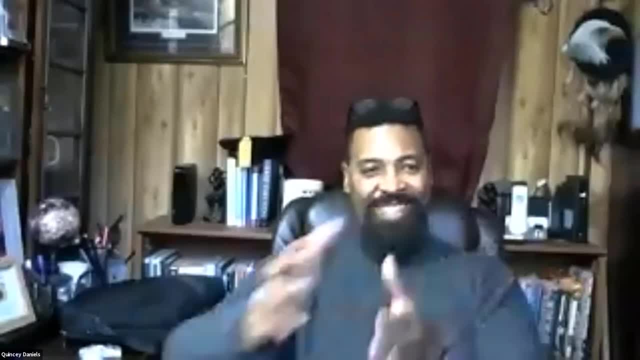 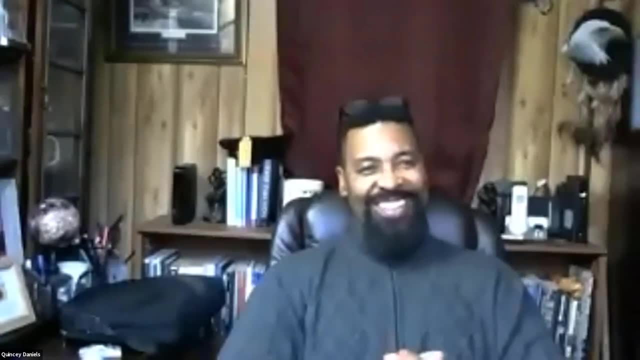 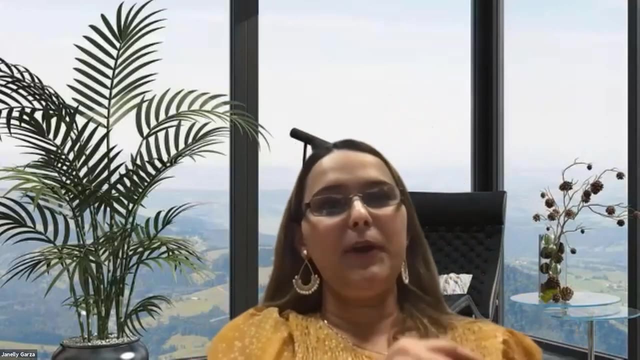 what's going on? how did you manage to get your codes and themes and kind of you know the encompassing part of it where it starts to jump out and say, aha, how did you do that? yes, so, um, I did that by going interview by interview. uh, the beginning step where I looked independently at 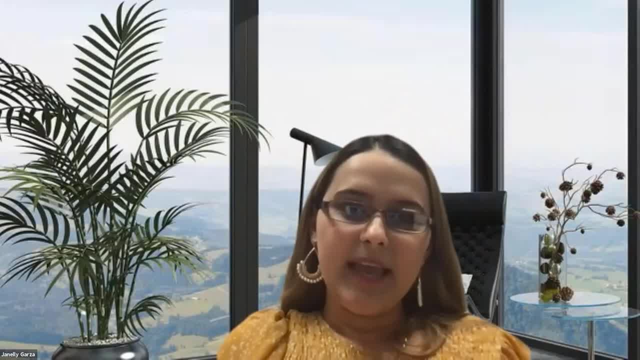 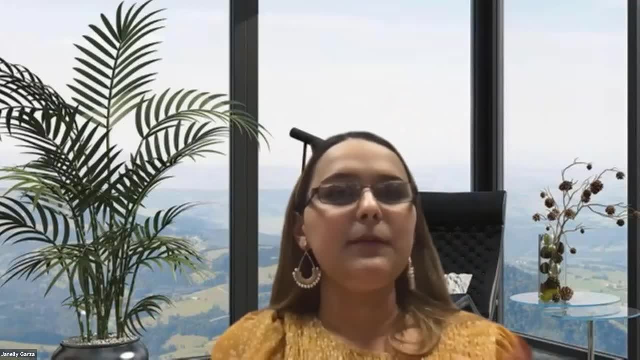 each interview and wrote notes on the post-its. and then I read the second interview and I wrote notes. I read the second interview and then I read the second interview and then I read the second, the third interview, wrote notes and started noticing as I was reading the different things. 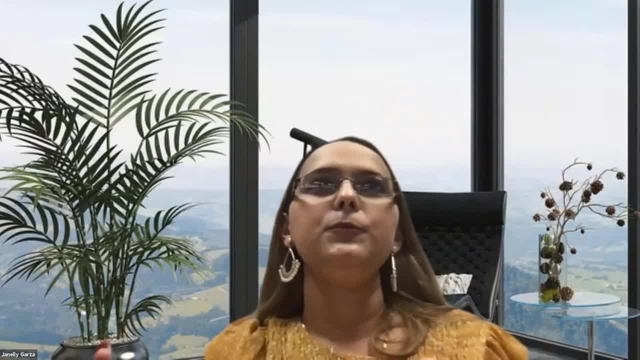 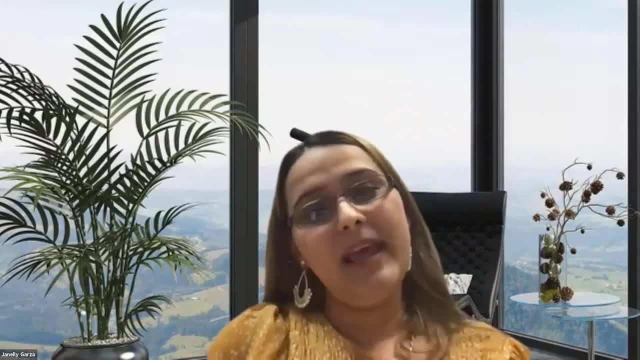 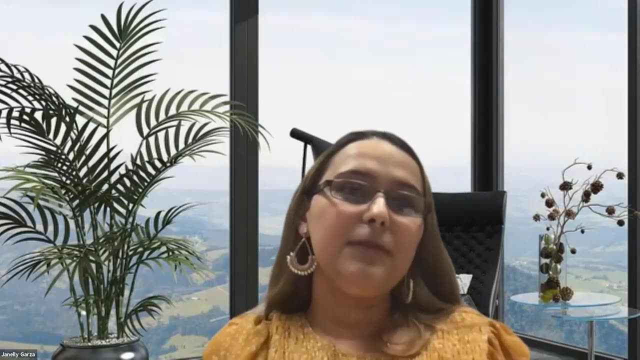 that were being really repetitive. the things that I found were emerging from from the findings, and that's how I started to create my codes. that's where they came from, and then, once I looked at all 14 interviews, is that I went ahead and created the questions for the focus group session, which 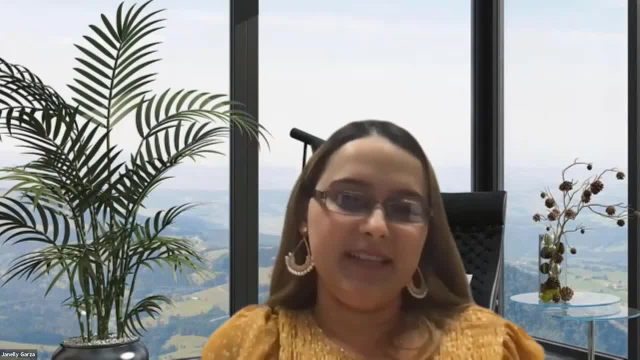 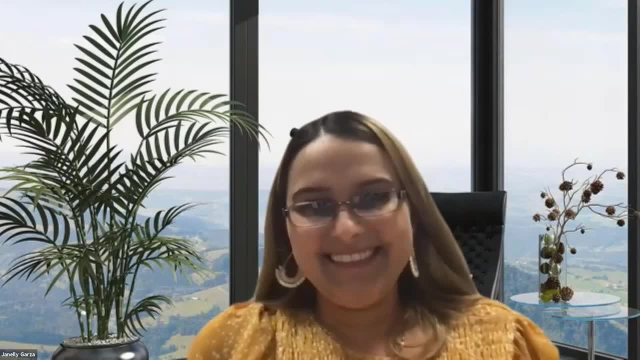 were more specific in what had emerged from those 14 interviews, and that's how I'm more or less motivated to be able to reach the target audience and just to get them to know me as well and be able to make a progress that way. so it's complicated sometimes, um, but in some instances, when I get 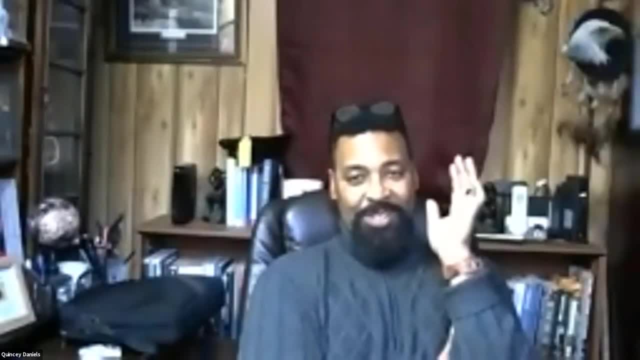 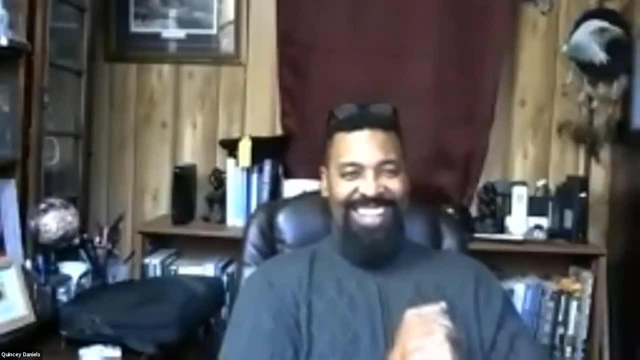 an opportunity to write a quote and I read it. I'm like, okay, I'm ready to write it and that's how I started. that I learned because it was hard. yes, okay, all right, thank you, I always had that idea. it's like: okay, I gotta, because I'm pretty visual, I always had to like connect stuff. it's. 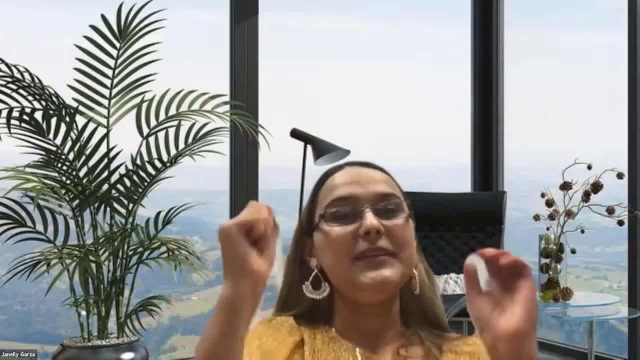 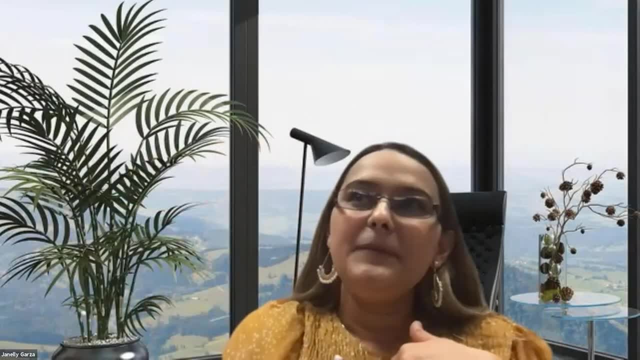 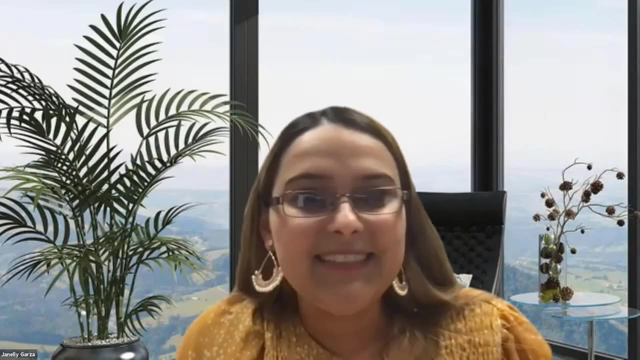 like: okay, otherwise I would forget by the time I read the third transcript. so okay, all right, thank you. so making my my notes was very beneficial, yes, being very intentional about each question. So now, I'm sorry. how did you transcribe your transcripts originally? 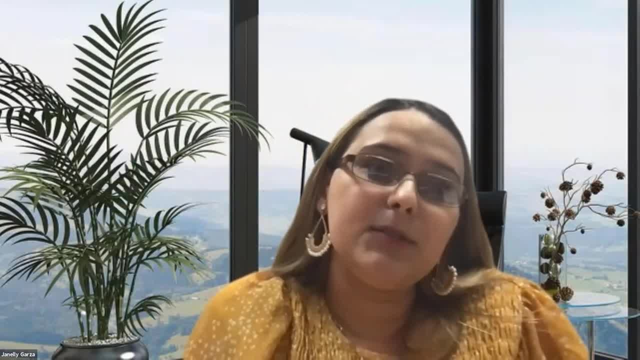 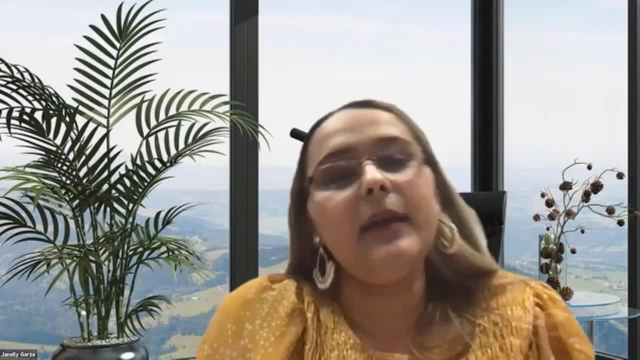 I used Otteri to transcribe the transcripts. So in my IRB I did ask for permission to record through Skype and to well, video record through Skype and to record through Otteri, And as I was doing the interviews I had my Otteri on my phone. 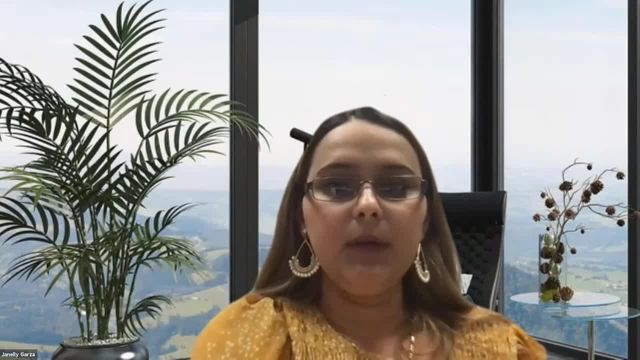 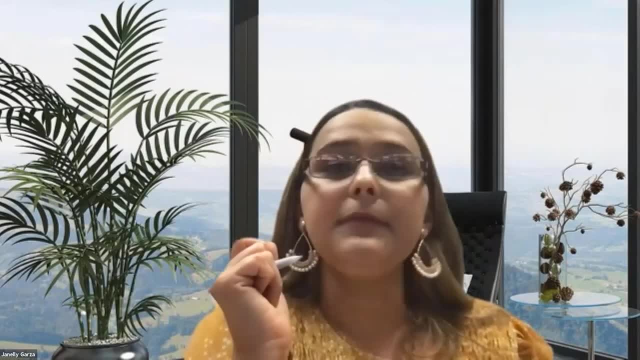 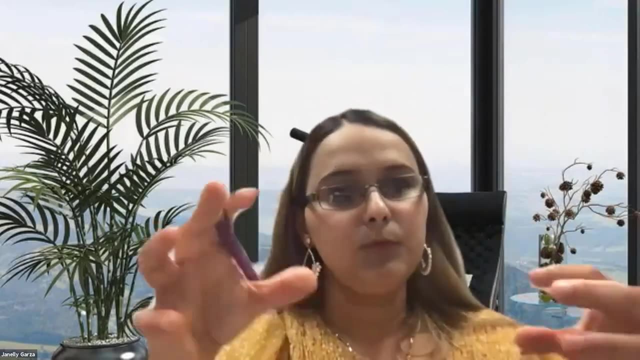 and I was recording, so I could have the visual through Skype and then the voice through the Otteri, And it's a very neat app. I did have to go back, though, and really listen again to the interview and some of the words, because we're Hispanic, we may have an accent. 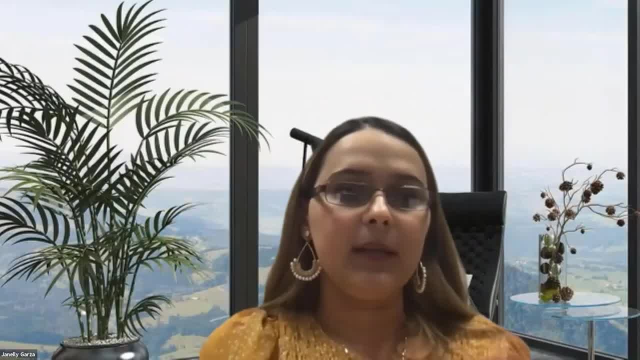 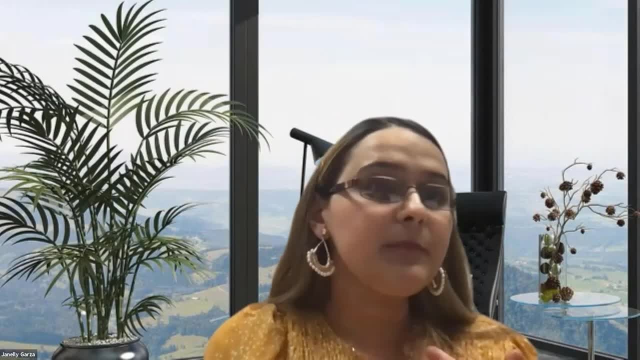 we speak in Spanish. I did allow my participants to speak in the language that they felt more comfortable with, And I did have to go back and change some of the words that had been spelled, misspelled or just pronounced in the wrong way. 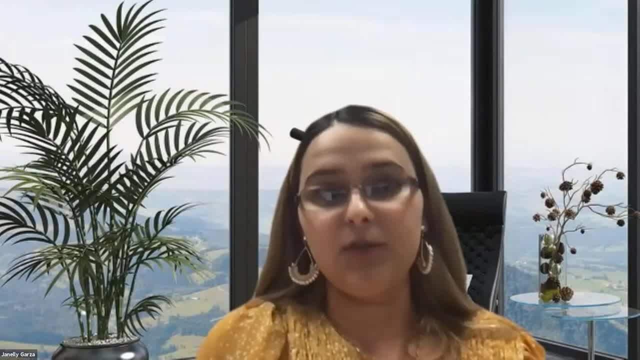 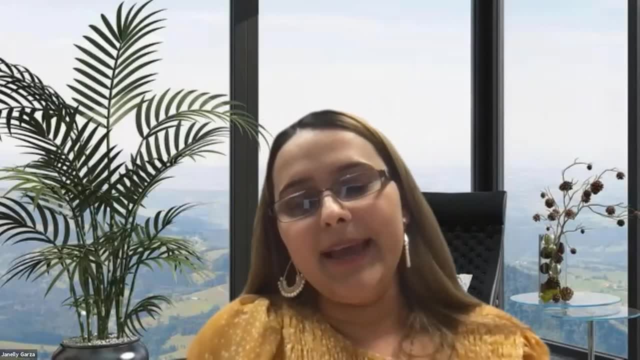 Yes, thank you for sharing. Yes, Otteri, And that's how I did the transcriptions and it was very beneficial. I see here that how did you connect with your interators? Again, I do have to give Dr Bloomberg credit for that. 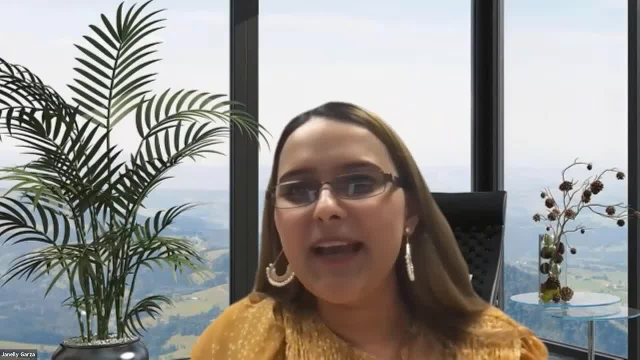 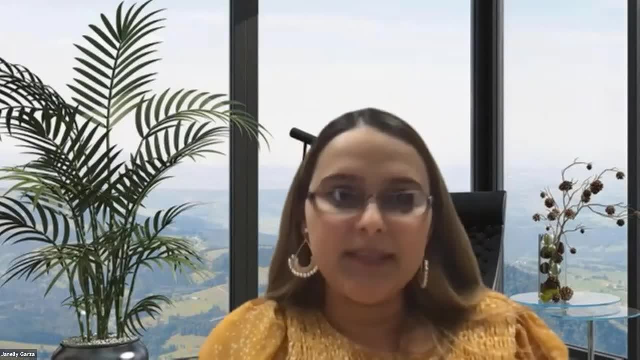 because I know Sandra Flores. I saw her earlier. Yes, she's here And I want to thank her Because Dr Bloomberg went ahead and connected us. We're both Hispanic. She lives in Puerto Rico, here in South Texas. We're able to understand each other. 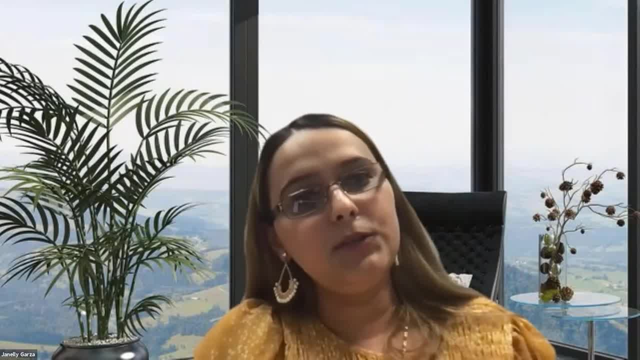 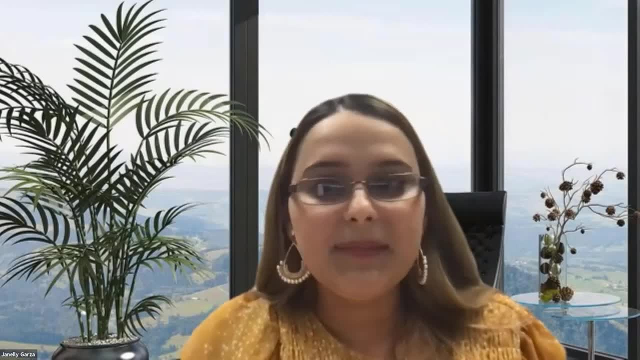 And that's how I connected with one of my interators. The other two interators are co-workers and they're currently getting their doctoral in education as well: Janelle and Sandra. I'm not sure if Sandra would like to just step in. 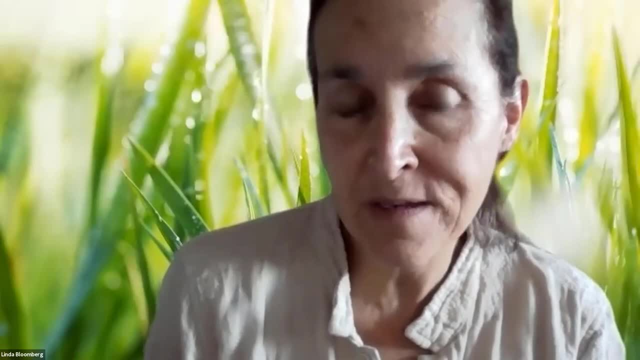 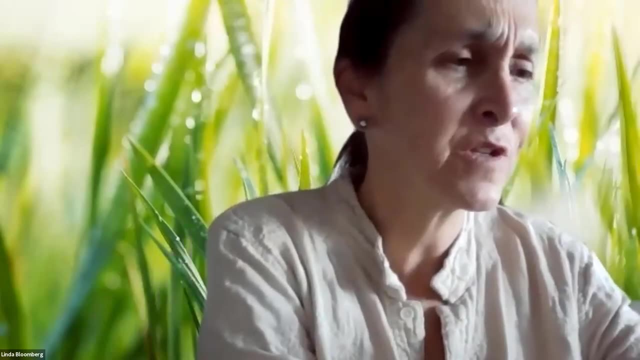 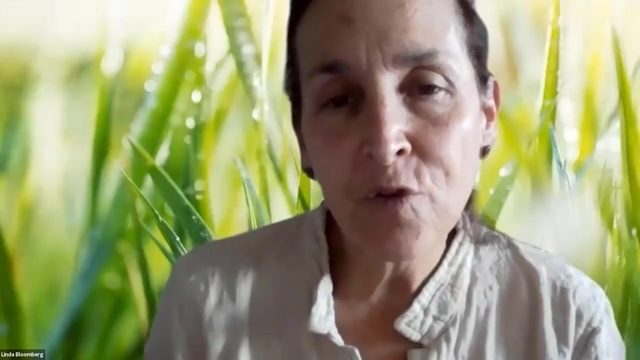 for a moment and just comment on her experience as an interator. as another, I'm a student in one of our School of Education doctoral programs and I'm also her chair. Sorry, sorry, that's a kid calling me. I don't know if you'd like to, Sandra, if you have anything to say. 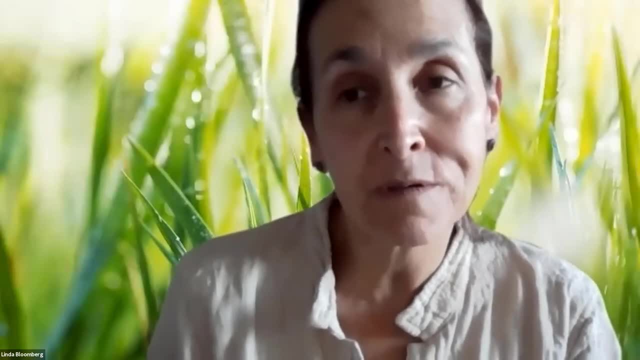 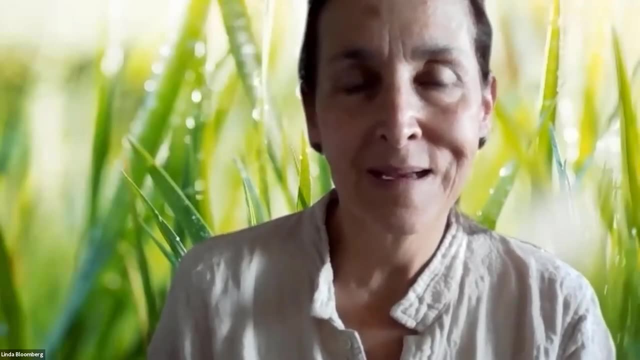 about that experience, what it was like for you, what you learned from it. Yes, definitely, Thank you, Hi everyone. Thank you, Janelle, for your presentation. Yeah, I participated in the program. I'm a student here now. 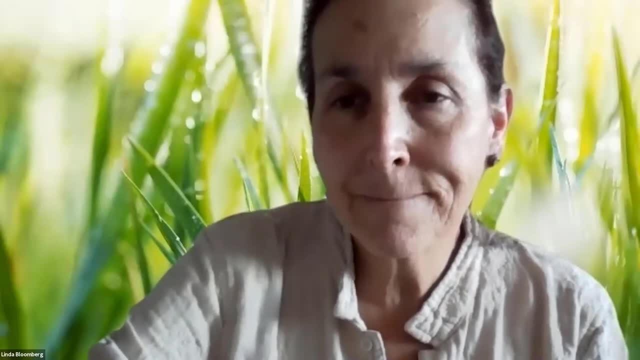 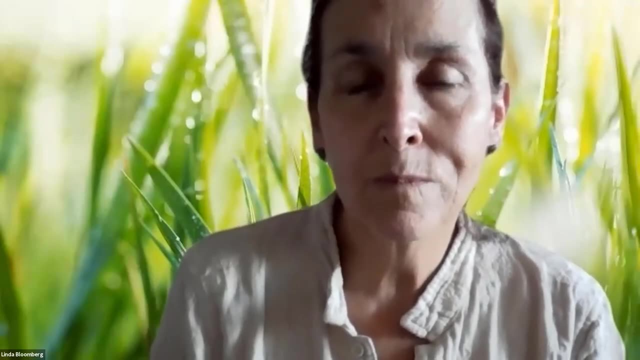 I'm one of our School of Education doctoral programs and I'm also her chair. I participated as an interator for Janelle's study and I really enjoyed the process, because I'm working on my chapter one right now, so I wasn't really familiar with the process. 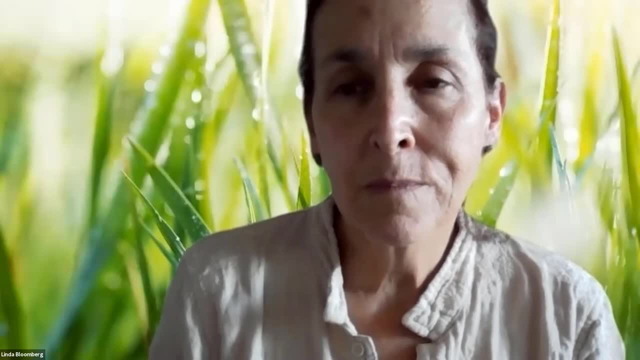 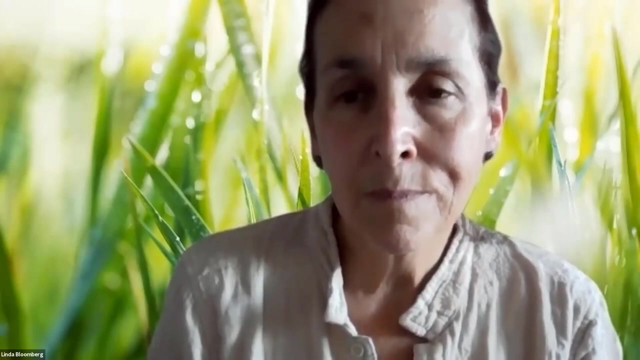 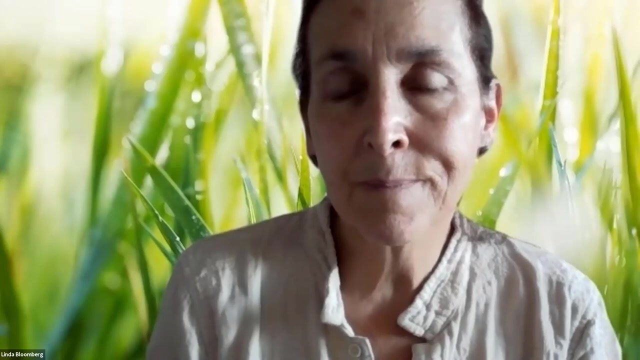 So I really got to enjoy to read every interview and really merge into the information and findings and just with all the data and learning how to come up with the codes and then themes. so it was a really nice experience just to get myself familiarized with everything and I found it really really helpful. 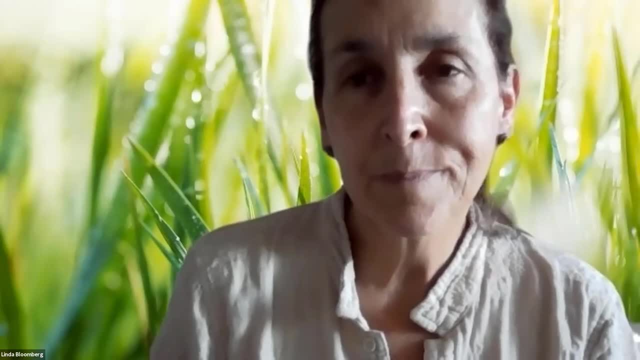 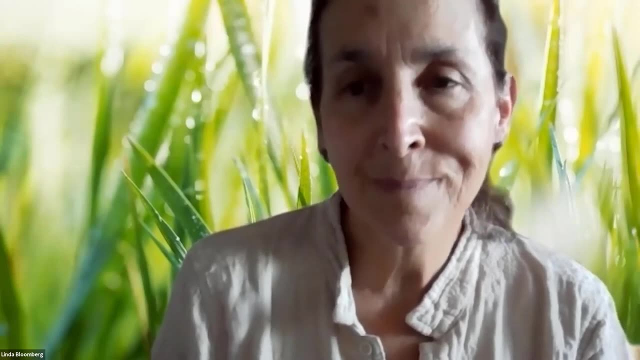 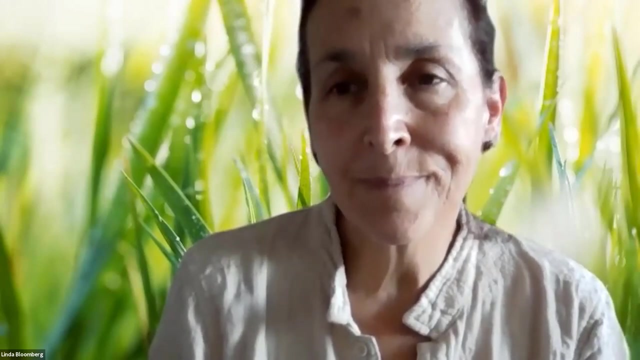 and I really enjoyed a lot of feedback from Janelle in you know, saying that we have to be very organized, and especially when the time comes for data analysis, I mean you're going to get so merged into the data like you have to. 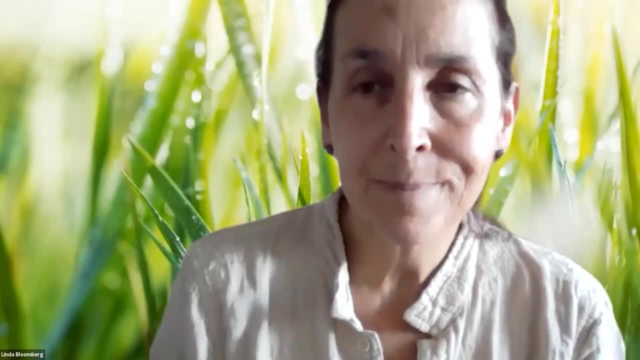 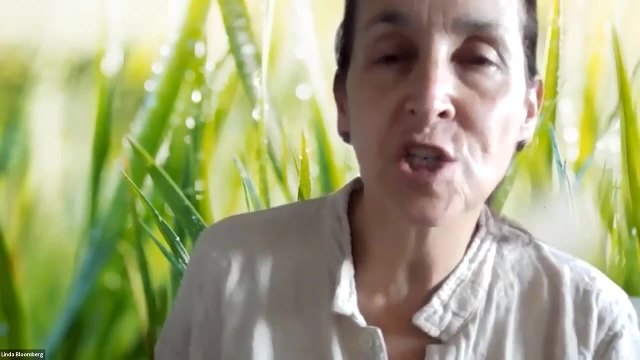 you know, be very, very organized and get everything in the right place. Yeah, and I just want to say also, my reason for connecting Janelle and Sandra, both of my two students, is they're doing research in kind of similar areas. 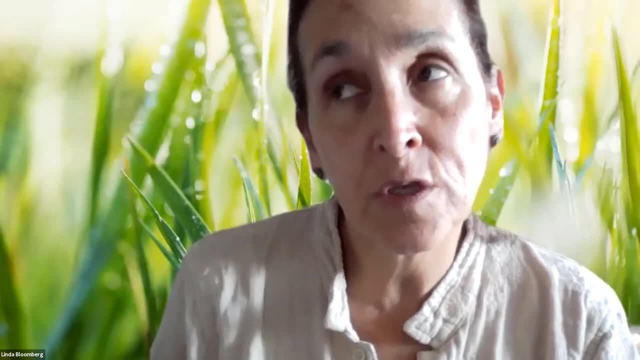 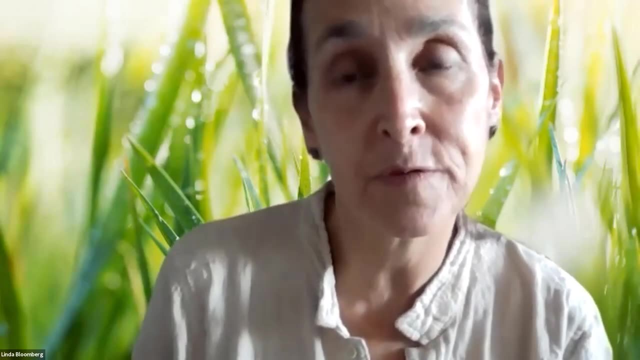 So, Sandra, maybe you just want to also just share the focus of your research, just so that the listeners can also hear that you're familiar with this area and that in your chapter one you've already started writing about this. Yeah, sure, definitely. 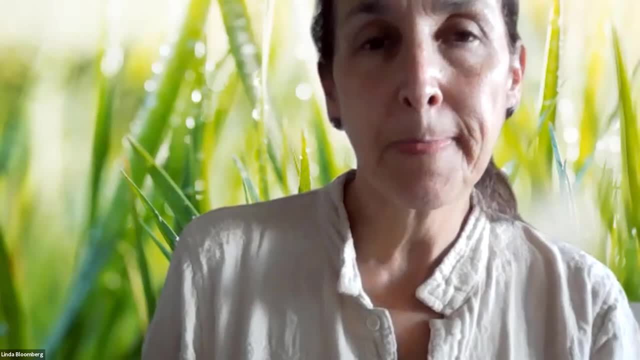 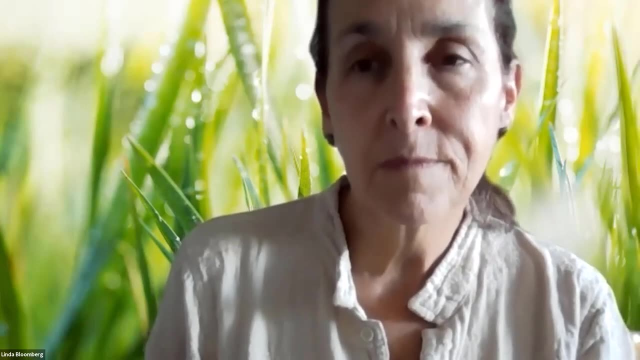 Well, I'm you know I'm. you know I'm a, you know I'm a. you know I'm a you know. my dissertation topic is about the limited cultural competence of higher education teachers who've been working with English language learners. 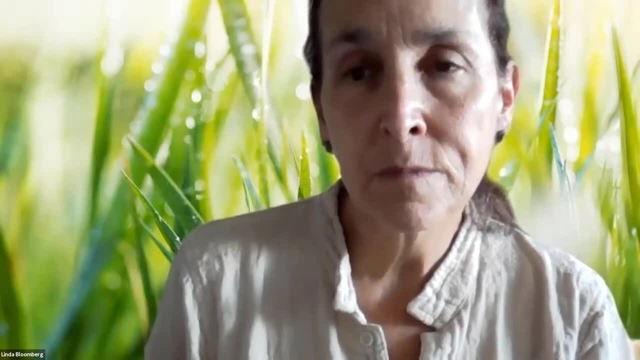 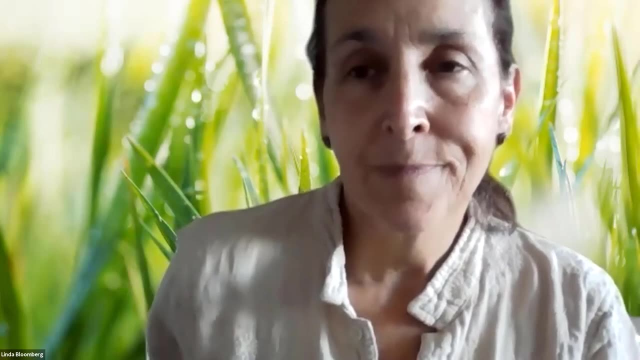 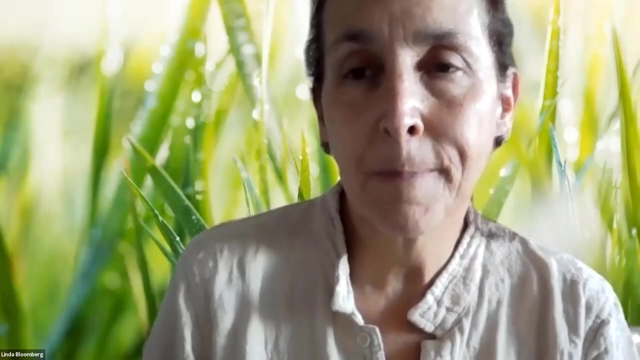 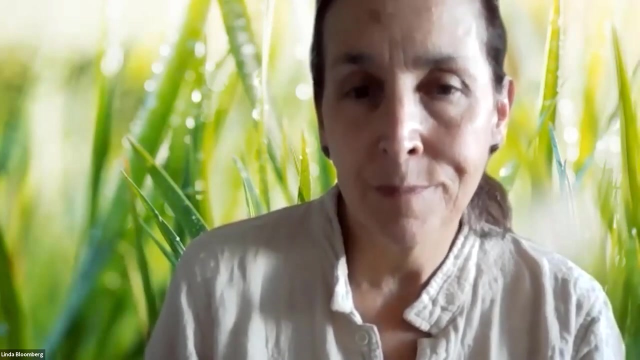 My topic is very similar to Janelle's, but her area is more in the elementary education, elementary grade level, and my topic is about like how prepare what the teachers are to deal with English language learners in general, because they all come from different cultures and, as we know, like 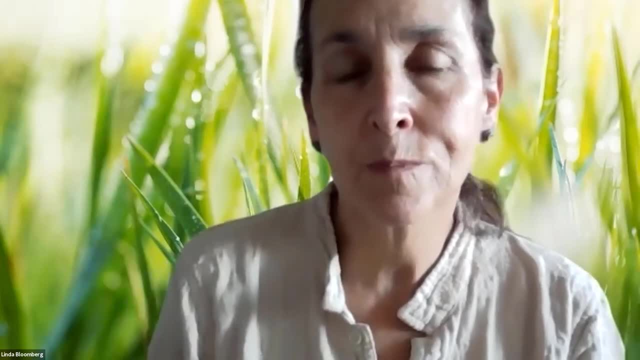 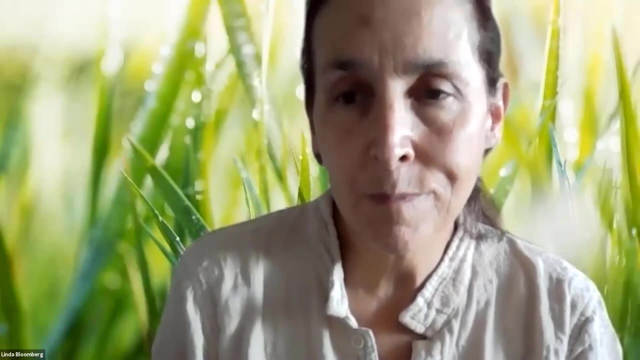 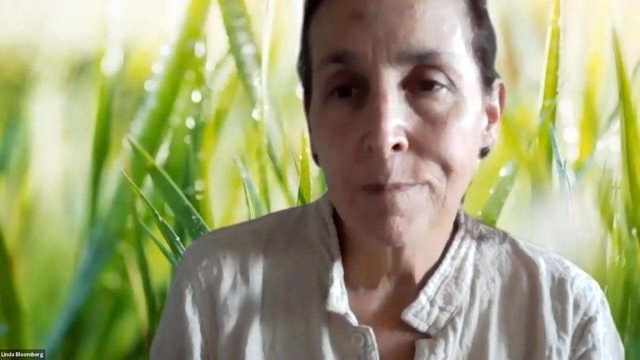 your culture dictates how you can learn a new language, So we have to really get teachers prepared on how to deal with the, with English language learners or just, you know, students who come from different cultures in general. Yeah, thank you. 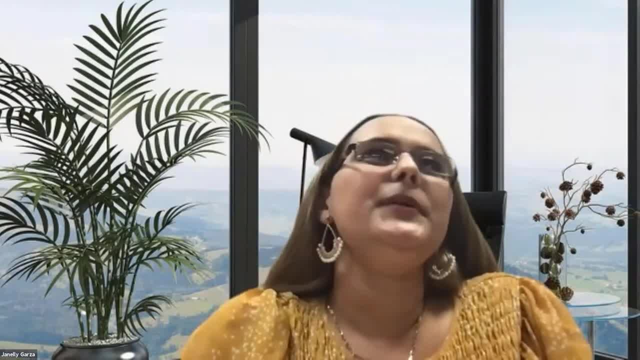 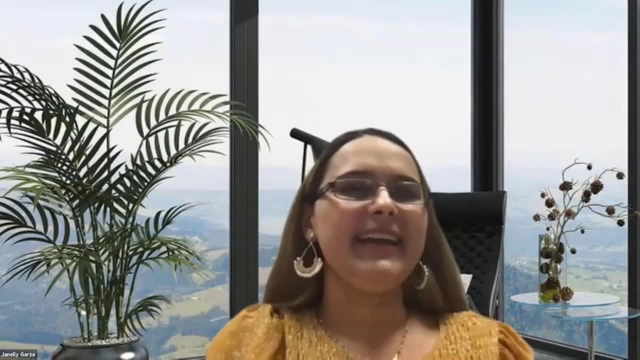 Thanks so much. Yes, And I do want to thank Sandra, because I remember I think it was a Sunday when we met through FaceTime to discuss the coding scheme and talk about her feedback and our conversation, and she was extremely tired. We were both very tired. 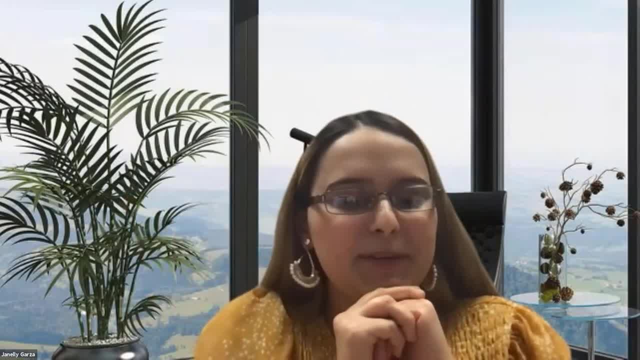 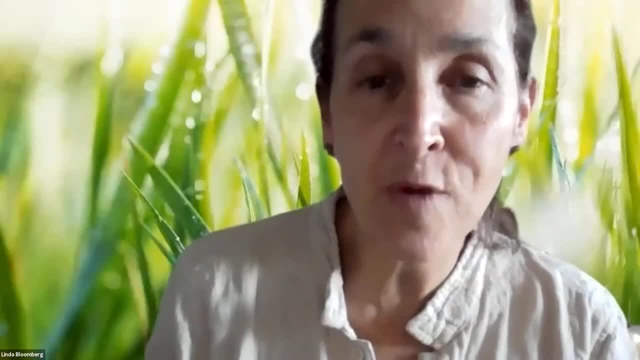 It was a late Sunday- And thank you so much, Sandra, for your collaboration, yes, and Dr Blumberg for connecting us, because, Well, I have to say, nothing gives me greater pleasure than to connect students so that we are all part of this larger learning community and we can support each other. 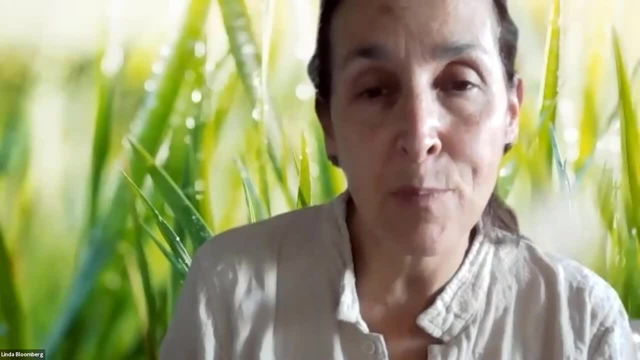 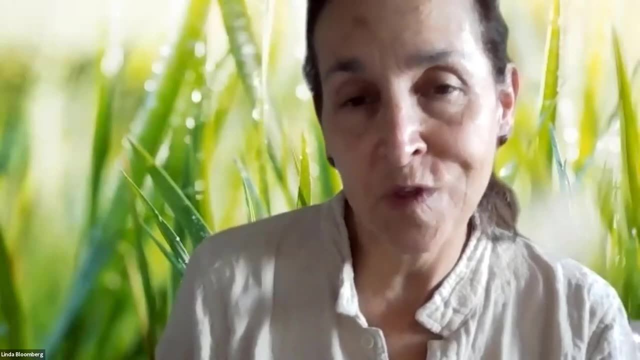 Yes, And I really am so thrilled that you were able to collaborate and I'm sure that you will collaborate going forward. and I know, Janely, you're a big inspiration for Sandra as she's setting off on her study on her Chapter 1.. 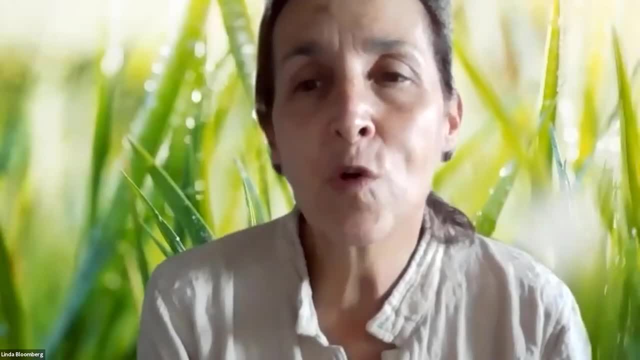 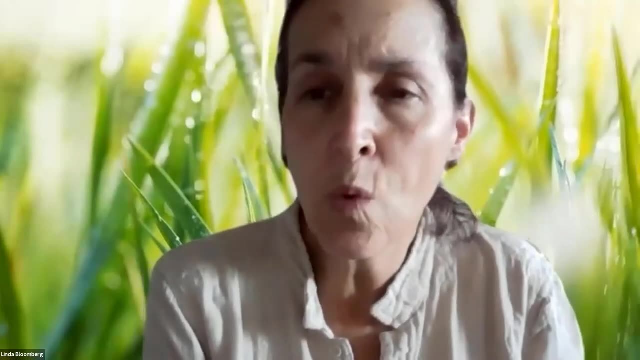 So what are the questions? thanks, Sandra. What are the questions from anyone in the audience? I see there are some of my other students in the audience. faculty members, What pops out to you that you'd like to ask, Janely? 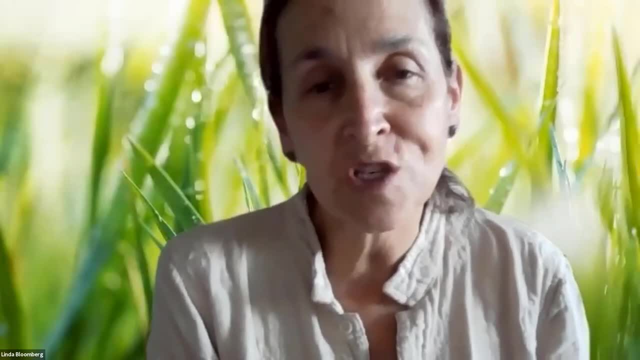 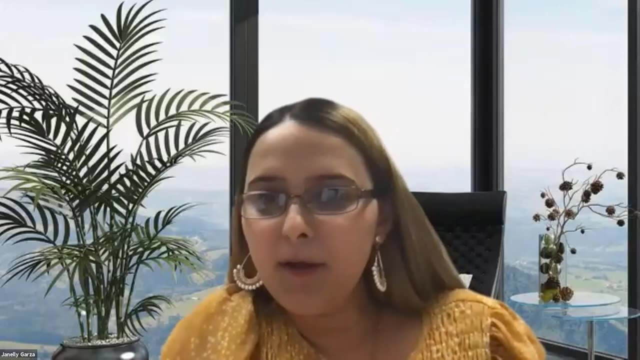 We only have like another five to ten minutes left and here she is and she's ready to answer any of the questions and share some of her strategies. Yes, I have one on direct message, Dr Blumberg, about member checks. 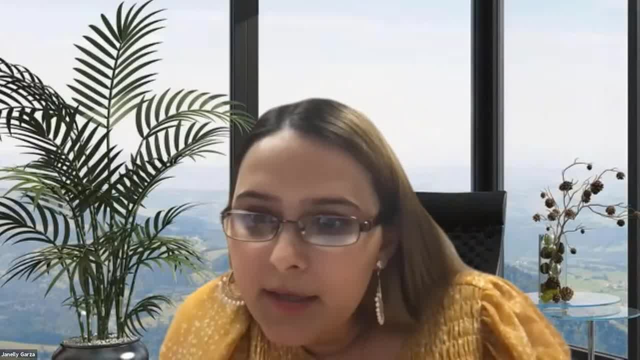 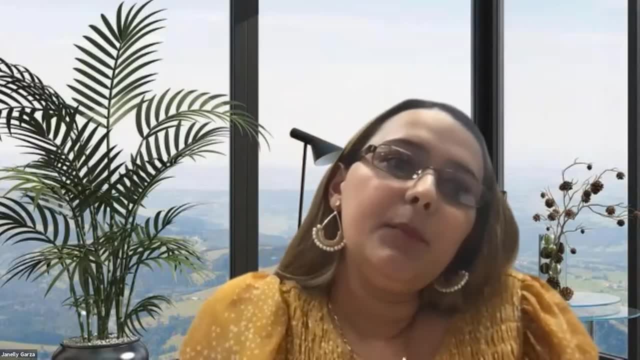 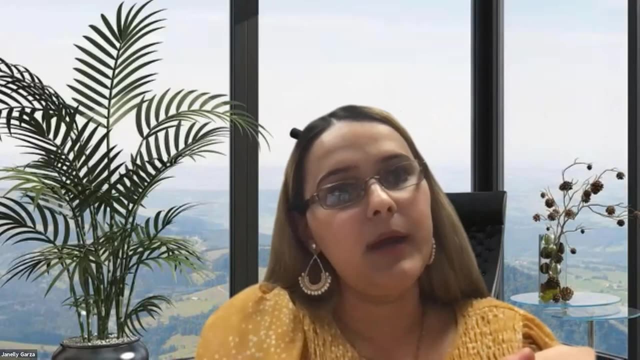 I did conduct member checks. Did I experience any special challenges in that part of my data analysis process? Not necessarily, because that was done prior to conducting my data analysis. I did provide the transcripts back to my participants and they did their member checks, so yeah, 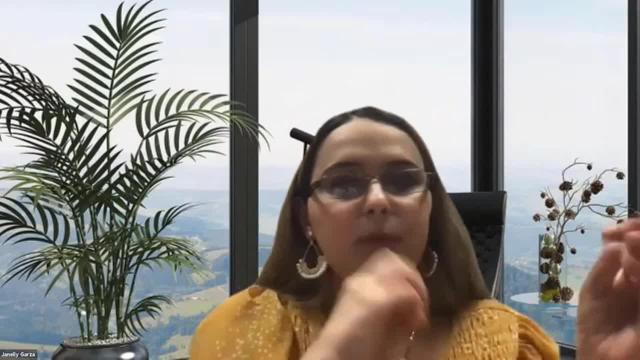 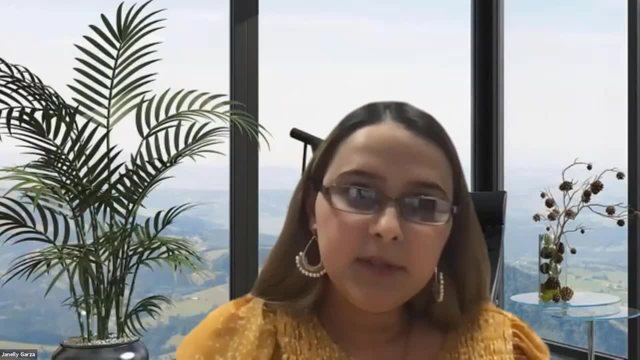 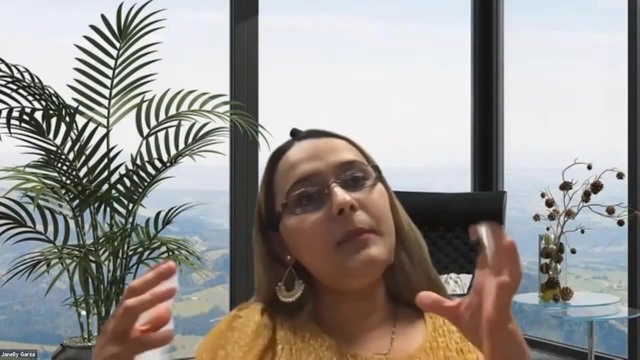 All right, member checking in that sort of this is what I would like to change. This is what is. it's fine. Not 100% of the participants replied with a member check, but I did include them prior. Now I have not sent them yet so that they can review my findings. just because I want to finish. 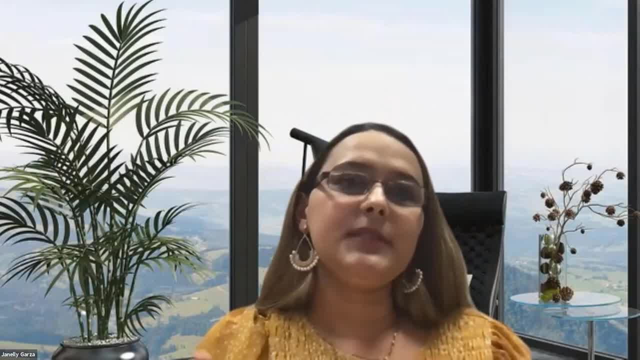 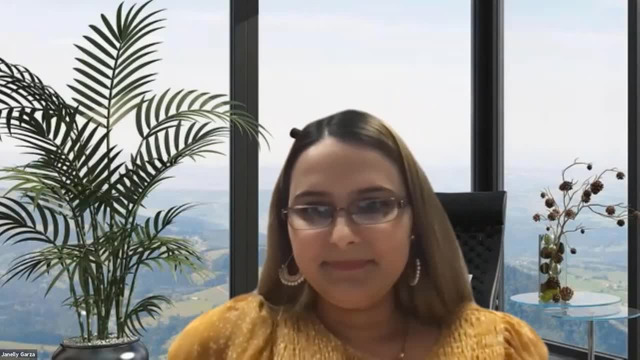 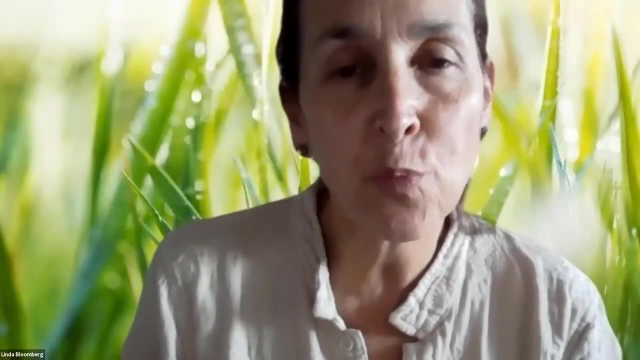 everything and have something consigned and well revised before sending it back to them. Does anyone have any questions for Janelle about some of the tools that she used, like the data summary tables, the interpretation outline tool? I know they're in my book, but Janelle 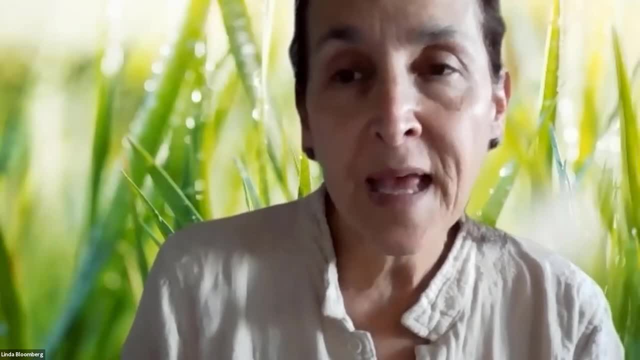 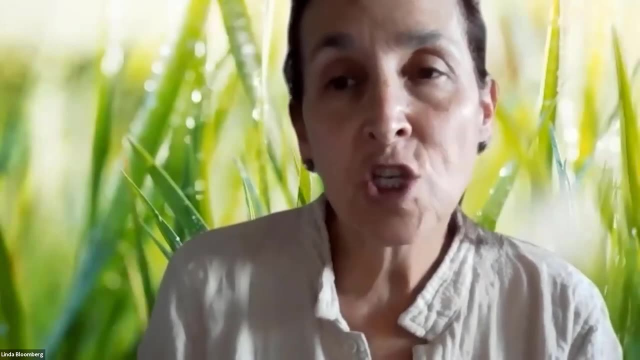 took the initiative to actually use them and she, you know, she then recreated them. So, if you take a look at her data summary table, she customized it for her own study and she, you know the way that she color-coded her focus groups in red, as opposed to her interviews that were in black. 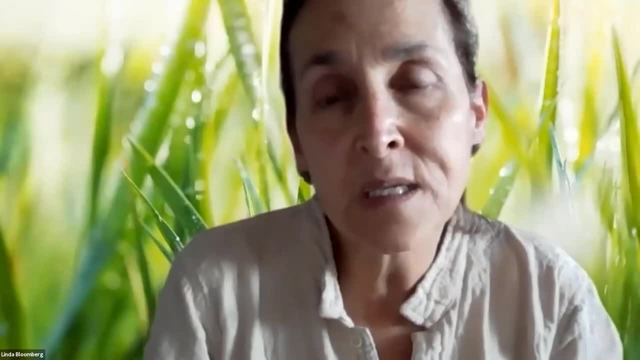 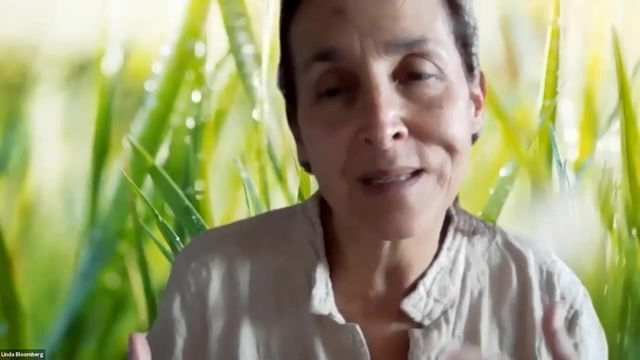 and so she could see where there was alignment and where there were similarities. Are there any questions about that that Janelle can share with you, about how she actually came to do it? Because, as Dr Daniels pointed out, it's such a huge process. You landed with so much data. 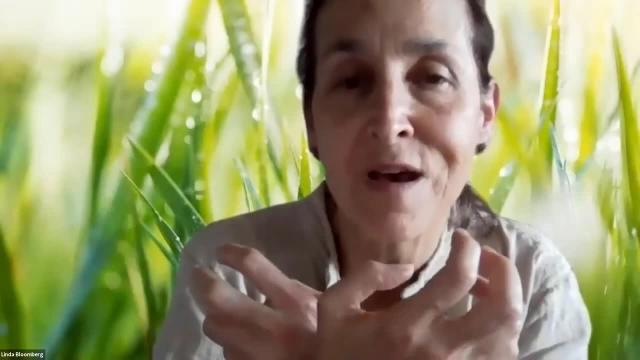 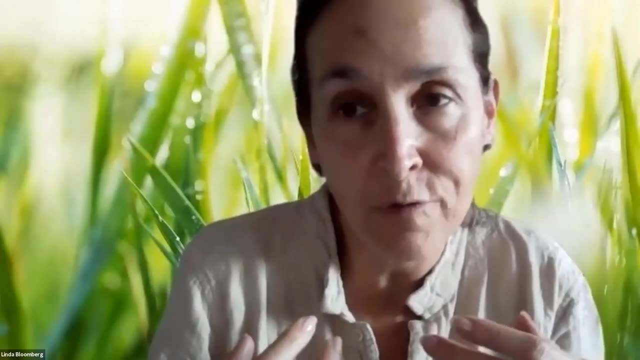 and now you've got to sort of make sense of it all and put all these strings together. and Janelle did that with all of these different tools and strategies and so much hard work and dedication. It just doesn't happen overnight, Janelle, maybe you can also just tell everybody. 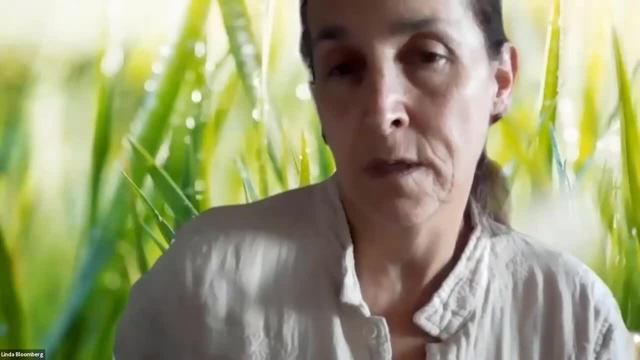 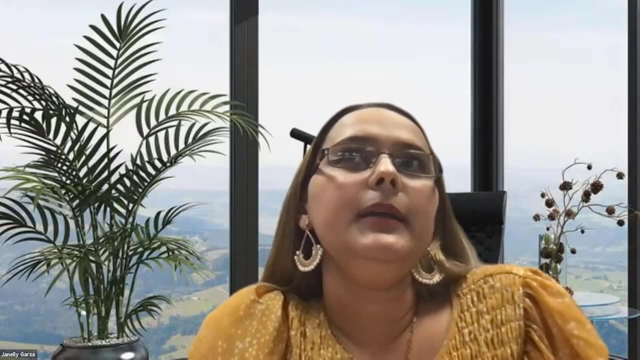 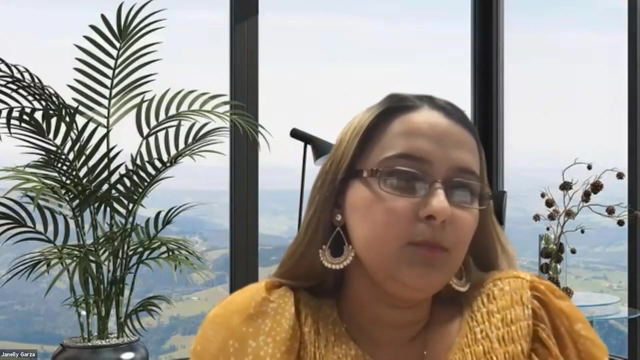 how long you'd have spent on the data summary table, This whole process. It's been a while, I think, from when I started collecting my data. It was back in March, and then we're October. I did start writing Section 3, I want to say maybe July, August. 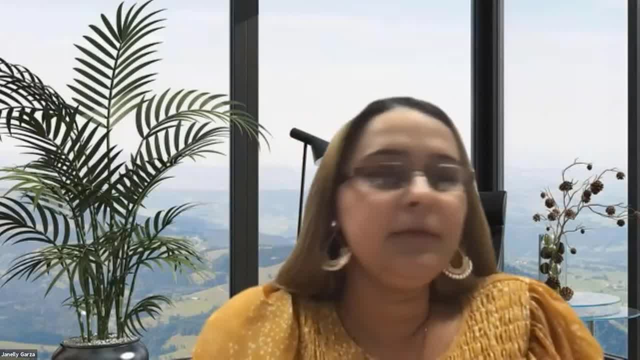 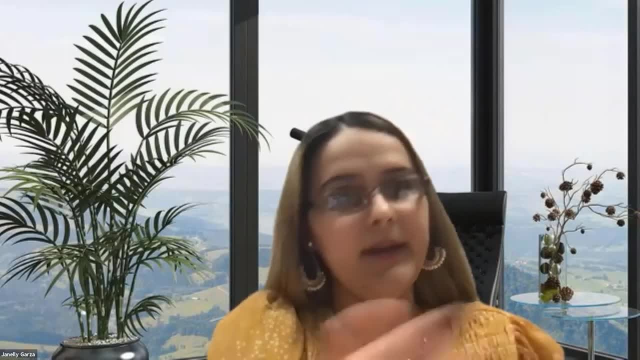 more or less and I'm still not conforming myself with. I'm just going to connect to any research that connects to my findings. but, really, being specific, I'm not going to be specific and intentional about what I really want to entail because, again, 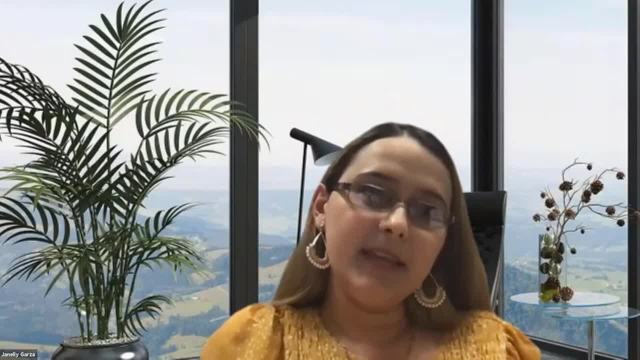 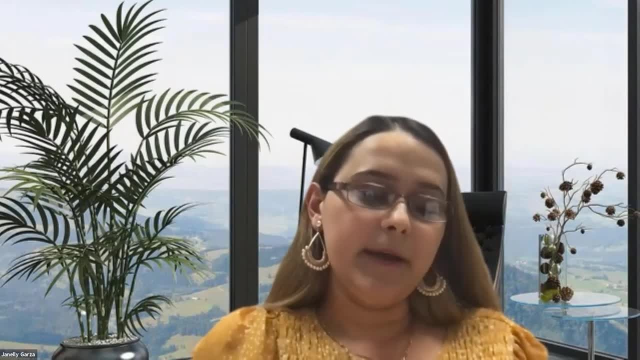 it's our work that we're presenting to others, but it has taken a long run. I know that some of the challenges that I did experience when I was collecting my data was that, since it was with teachers, we were doing virtual teaching. It was during COVID time, so my entire study shifted a. 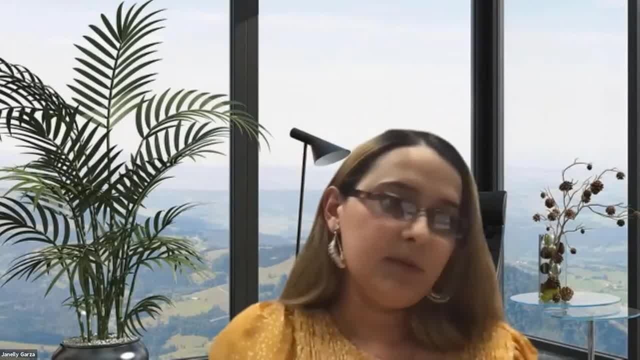 little because I wasn't able to do observations because I wasn't allowed to go in person. Teachers were extremely tired through the day. I was able to do observations because I wasn't allowed to go in person. Teachers were extremely tired through the day. 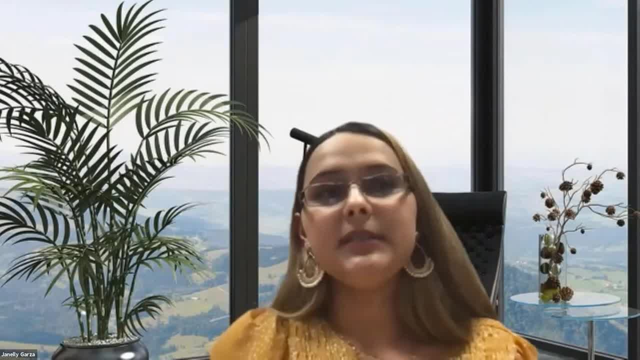 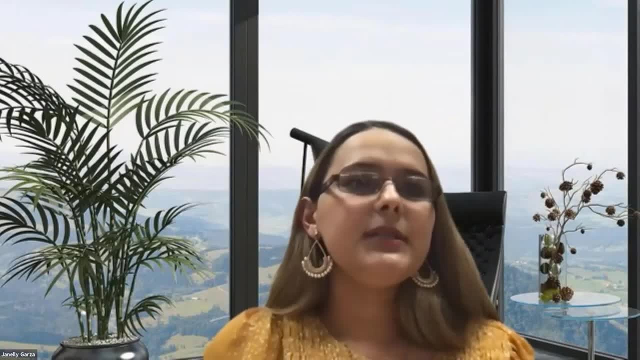 I was able to do observations because I wasn't allowed to go in person. The interviews were supposed to last 45 to 60 minutes. They lasted 20 to 45 minutes. Those are just little challenges in the recruitment process that I did experience. 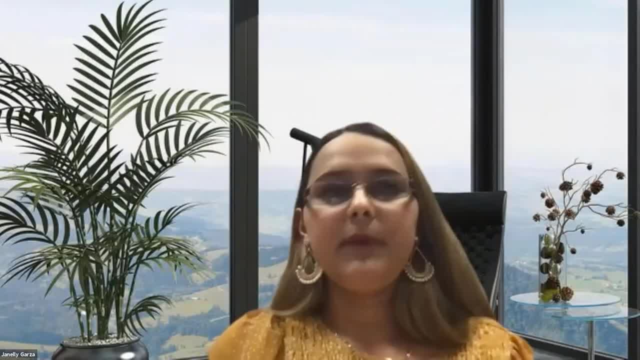 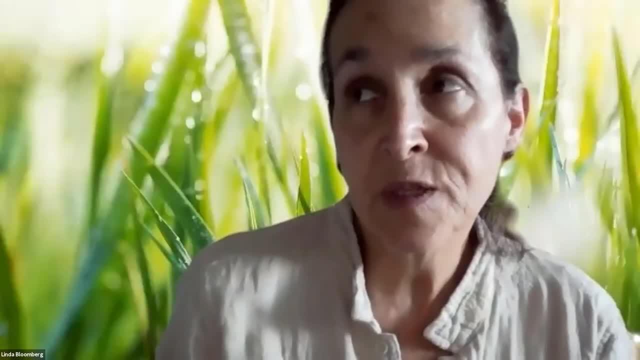 In the long run, just collecting my data, writing my findings. it's been a few months, probably six months. maybe I think you said it's been six months, but it's been six months of hard, solid work. It's not like Janelle has dropped off. She hasn't taken a break. 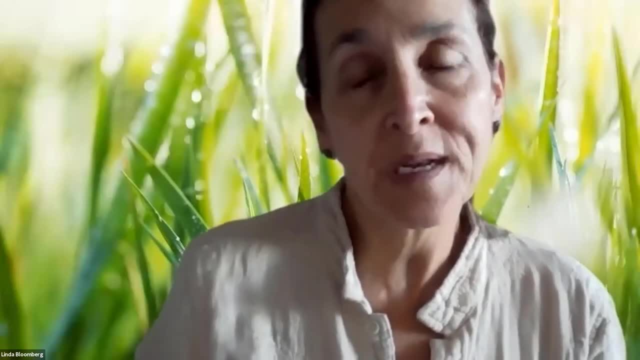 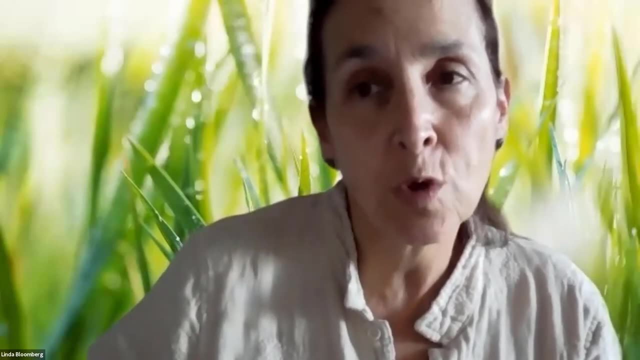 She's gone along with her courses. She's been an outstanding student in that she's taken not that many courses to get where she's gotten to, simply because she's worked really, really hard and she's had a lot of organization on her side that she set up. It didn't just happen out of the blue. 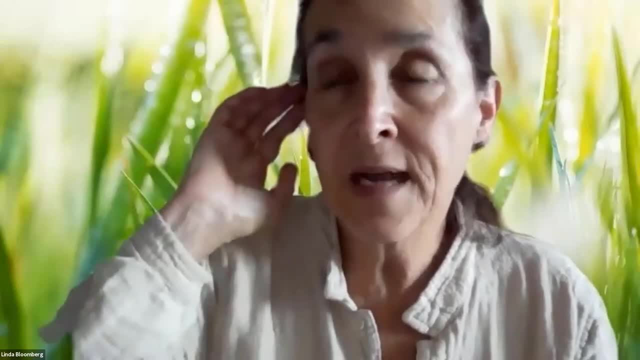 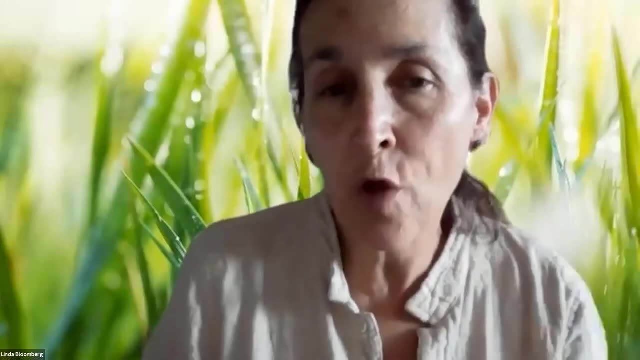 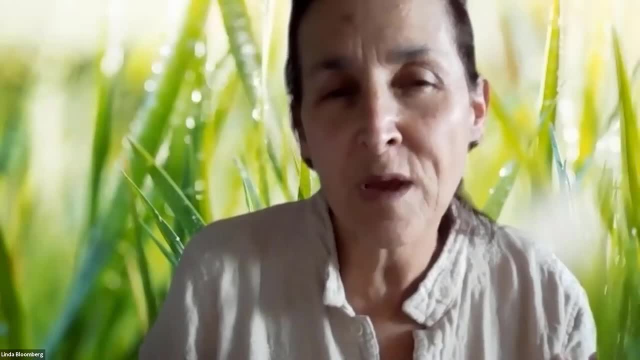 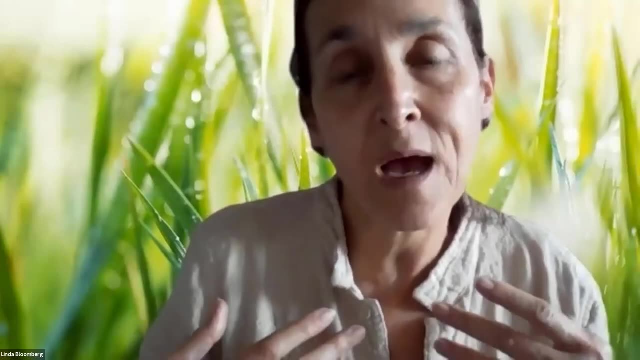 Create new data collection methods. I can't remember if we had to reapply to IRB. I can't remember if we had some little modification there. Yeah, we did. That's part of qualitative research. It is messy. I think Janelle is just a really good example, an excellent example, of a 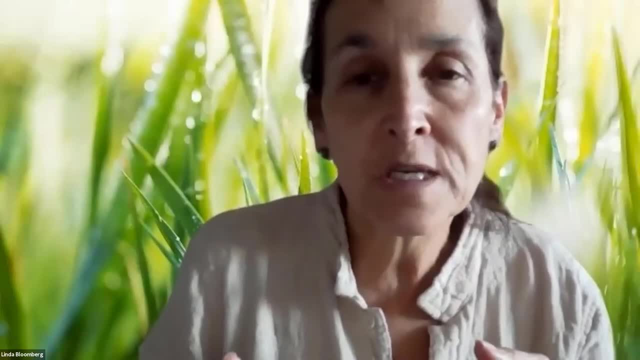 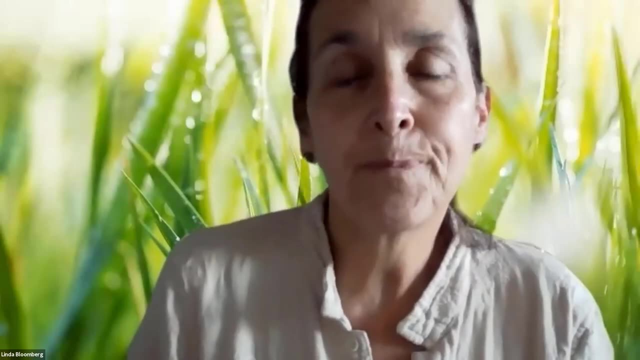 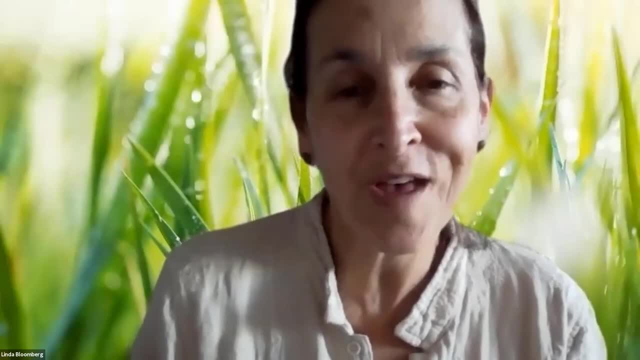 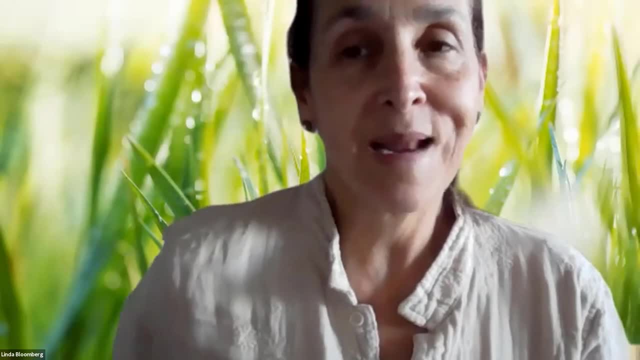 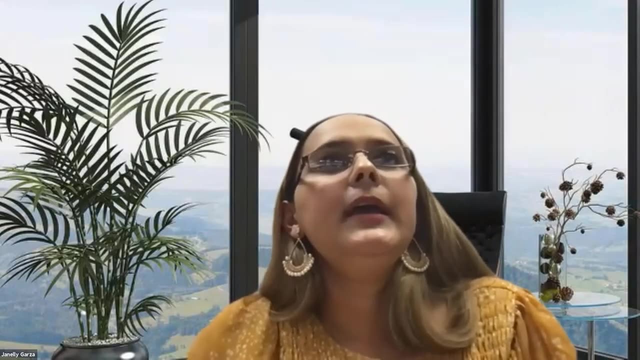 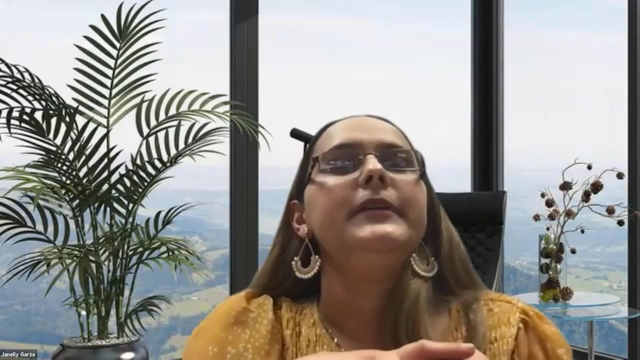 any questions for Janelle on that? maybe she can shed some light on her strategies. Yes, feel free to ask me. I'm more than happy to share. I do have a full-time job. lately It's been difficult because I was telling Dr Grinberg a few weeks ago. I've been having to work. 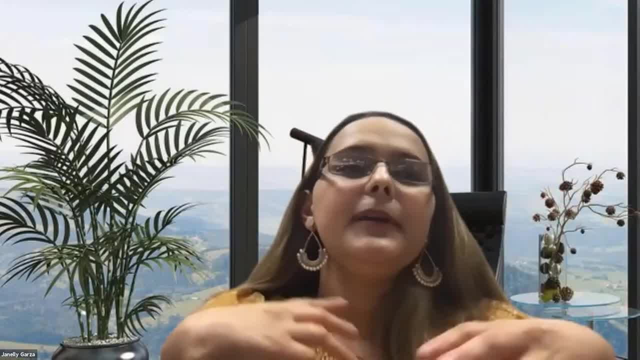 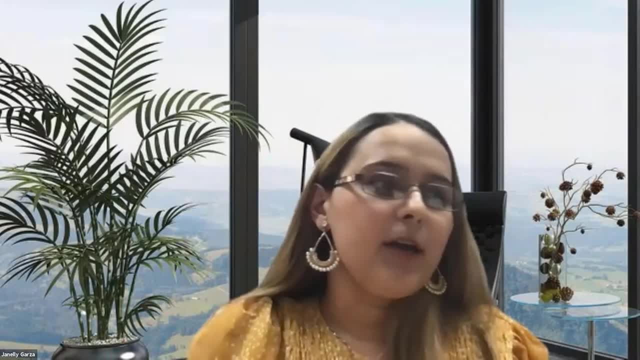 Saturdays I've been having to work until six. It's just becoming a little harder and harder to just really sit and in the back of my mind I want to sit and write and connect. so it has taken a lot of time, sacrifice, effort and organization, more than anything because 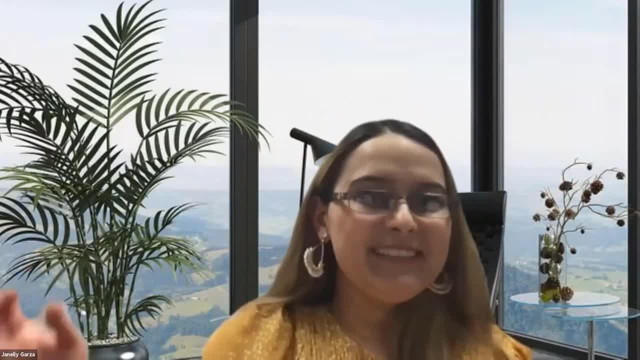 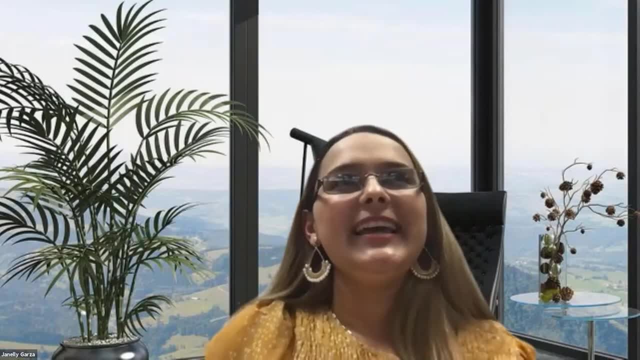 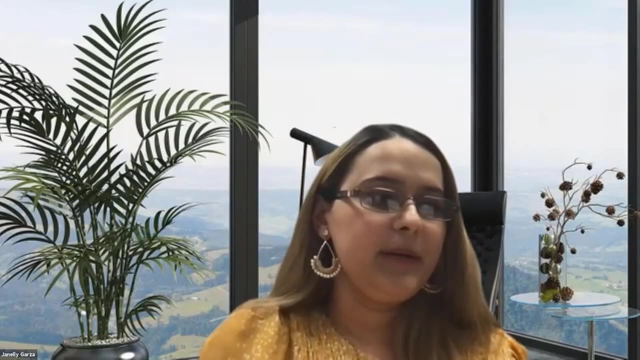 I remember telling Dr Bloomberg my goal was to graduate in September, to finish by September. no, not that it didn't happen because I didn't want to, but it's just that's how the process is. if I really wanted to do this work with quality, to to what, what I expected from myself, it was it's. 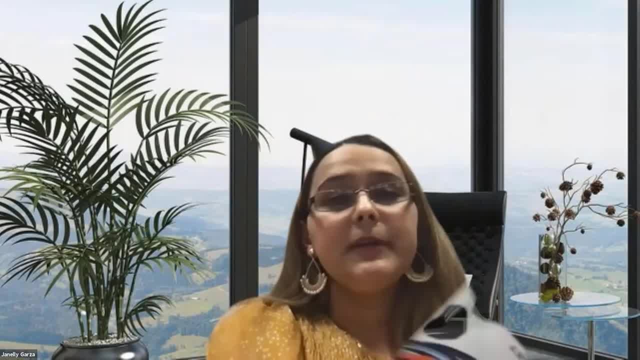 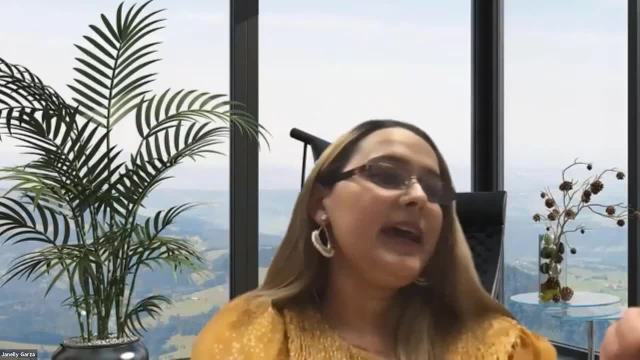 going to take longer. the resources again. the templates are already in Dr Bloomberg's book. she has a website. here's a book. she has the website and the website has all the templates there. they were a great resource for me to organize myself, more than anything because 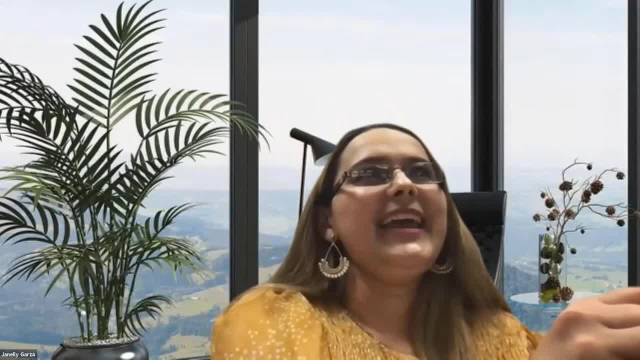 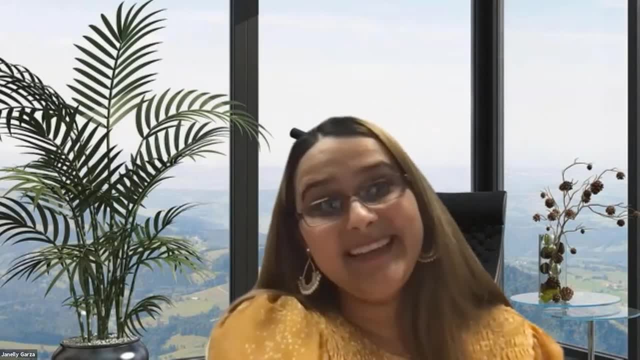 as you all can see, I started with post-its and then I kind of lost track of okay, who said this, who said that I found this data summary table. I'm like, okay, I'm taking it and I did make a few, make a few modifications, but more than anything. 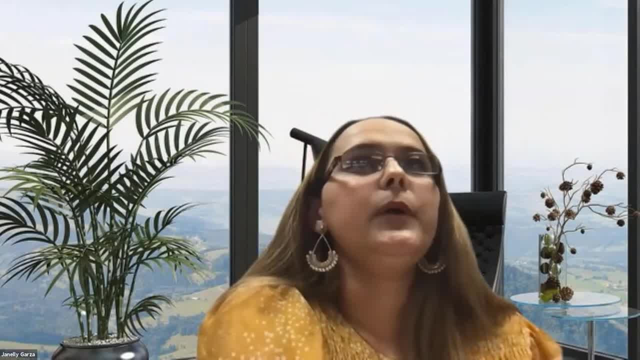 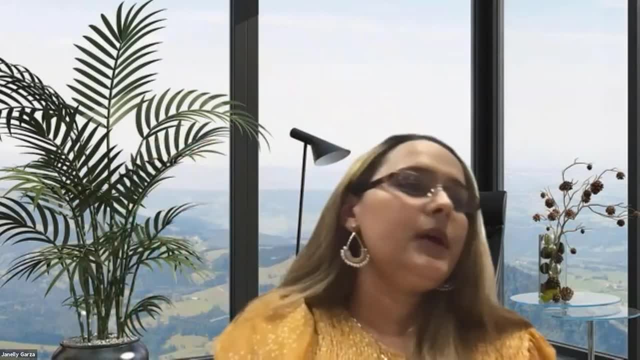 it gave me that visual. having that visual, that connection to where. if I'm questioning about my triangulation methods, well, you know what. this is how I try to eliminate data. I had the visual, I had the focus group. this was mentioned by different participants at different specific 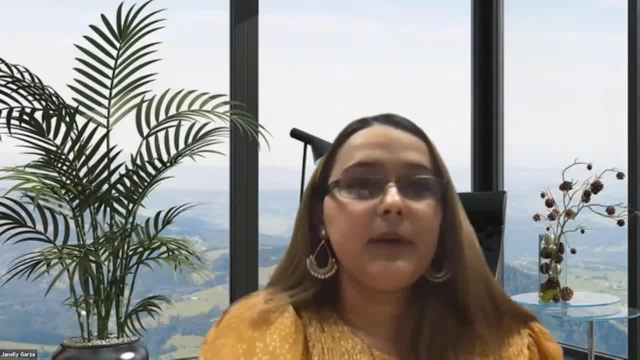 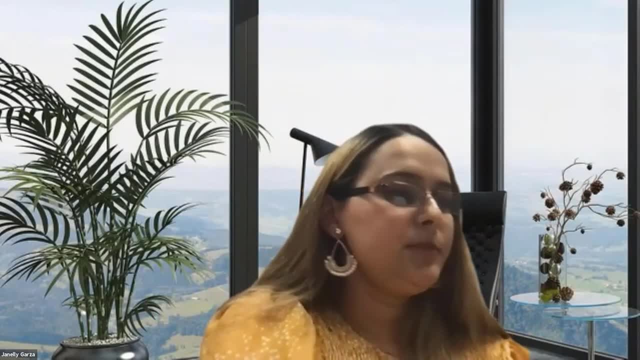 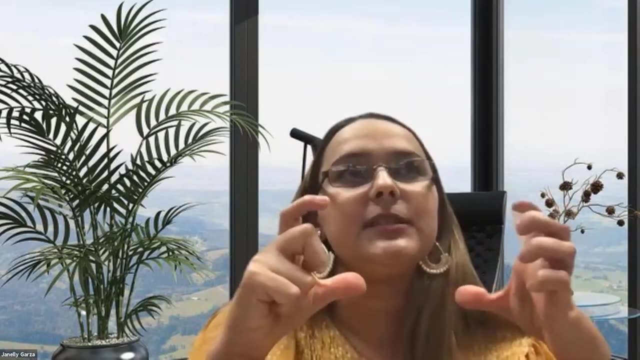 moments and it just really summarizes what everybody said. and even as I was writing my findings, I would reference back to that data summary table and because we have to put, for example, all of the participants or some of the participants, and we have to put, for example, some percentages- 90 percent, 75 percent of the 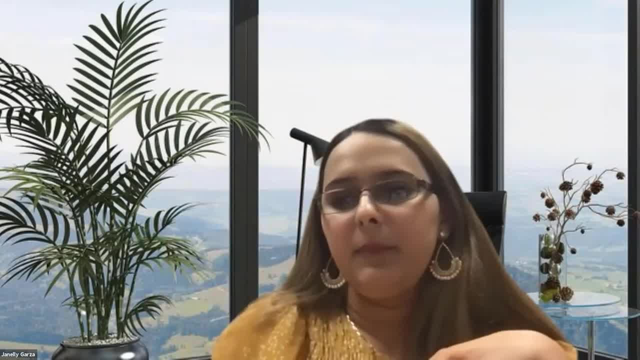 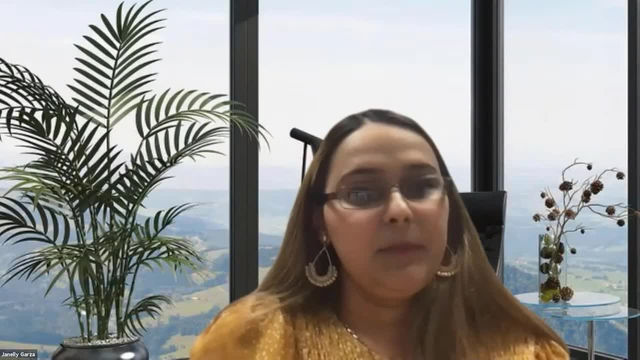 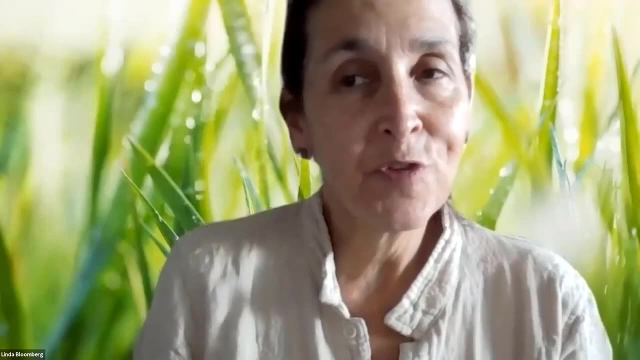 participants and that data summary table really helped me count how many participants had said what and then be able to jot down that percentage of with my, with what my findings had said. thank you so much. Janelle is up there. any few final questions? we have just a couple minutes left. 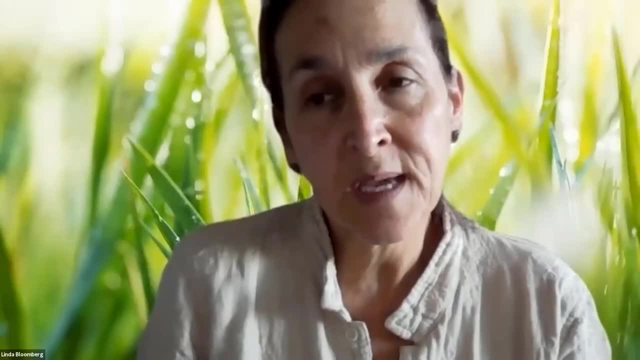 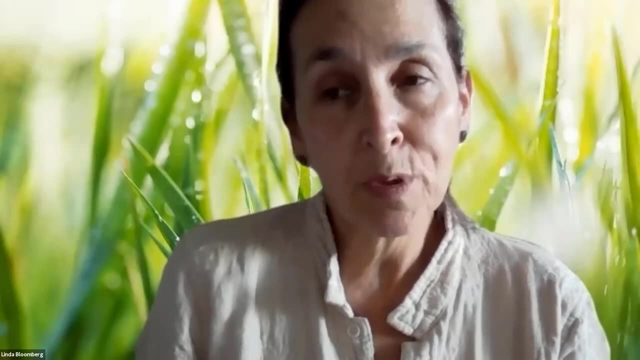 now I have to say I'm very, very grateful to Janelle for taking her time to present this and help others learn from the process, and this meeting will be recorded and posted so people can go back and listen to this and also share it with your peers, if you like. 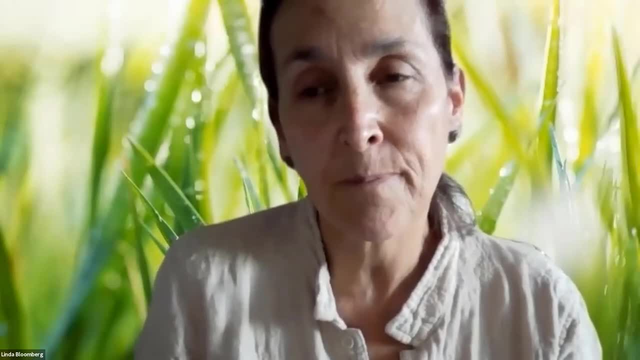 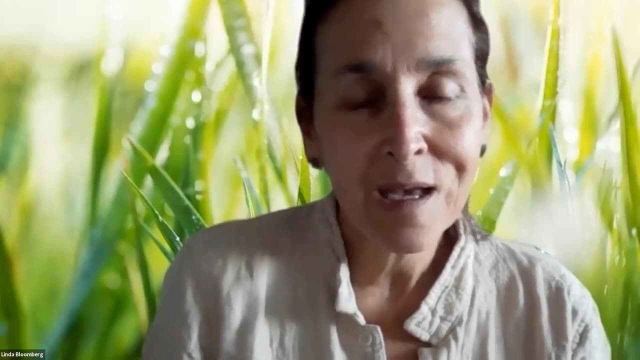 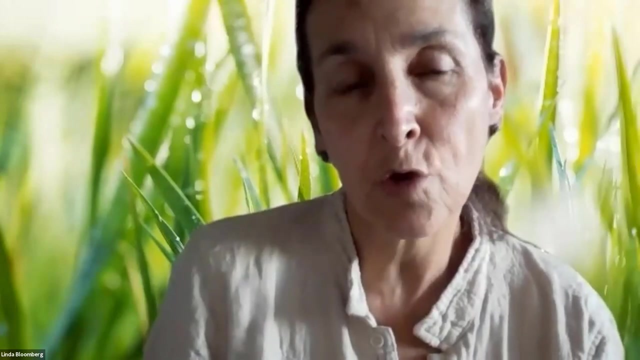 because it really is a very informative presentation on. thank you, Janelle. I see some clapping hands from Dr Daniels, from Dr Hayward form, Dr Beverly. it really was an outstanding presentation, Janelle, and thank you so much for helping support the brown bag initiative in our research, for our. 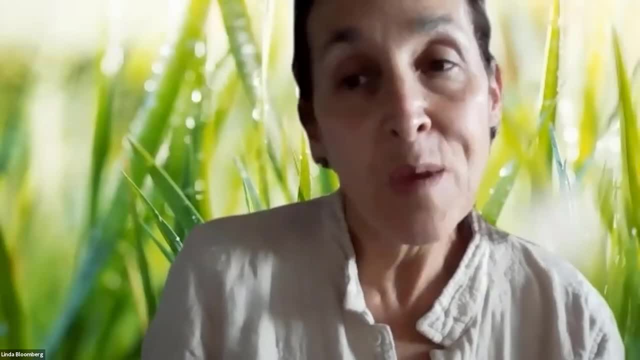 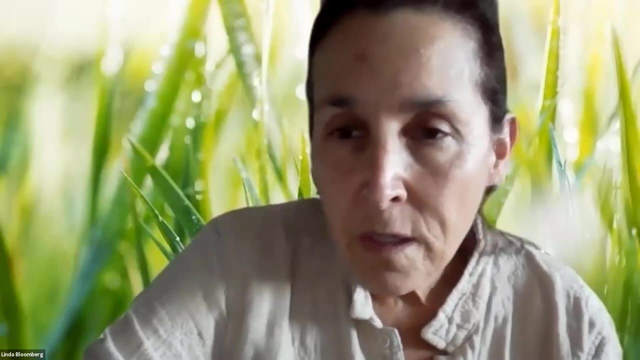 suggests, because yours fits very well within this framework. again, any other last-minute questions? is there anything in the chat? let me just take a quick look. yes, we definitely look forward to hearing you defend. so when Janelle is ready to defend, we definitely want to spot any response from a few people that are popular in the room, so I will hand over to you, Janelle, Please don't be53 so. I did as well, as I haveera said, to stop the screen. any other questions. we feel a little rescue. I didn't see through to any of our speakers groups. if there is any contributees and I don't need to repeat much, but just say thank you for having escrow and friend you and all the other sessions. 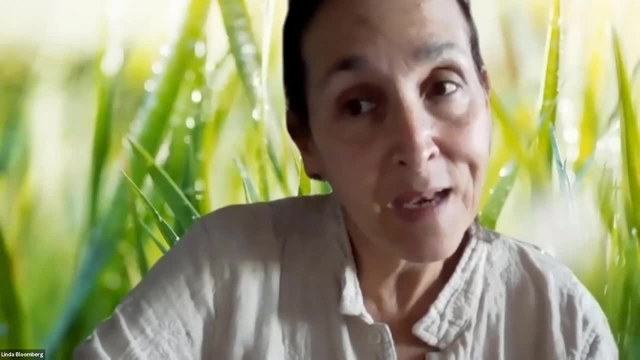 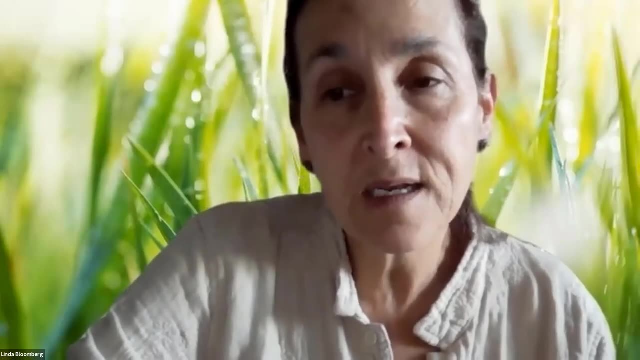 defend which is coming up, and she definitely will be graduating in the next graduation. I will let everybody in the committee know when her defense is if anybody would like to attend. And remember also, all of the defenses are always posted in the commons. 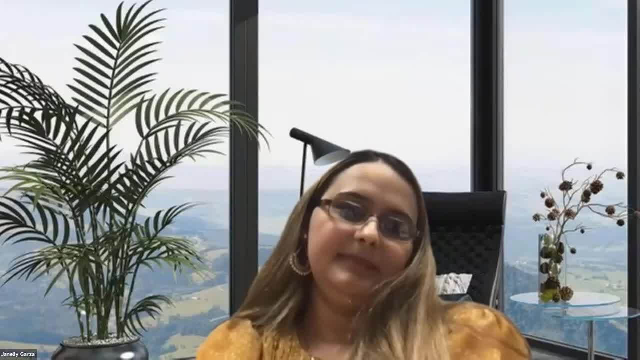 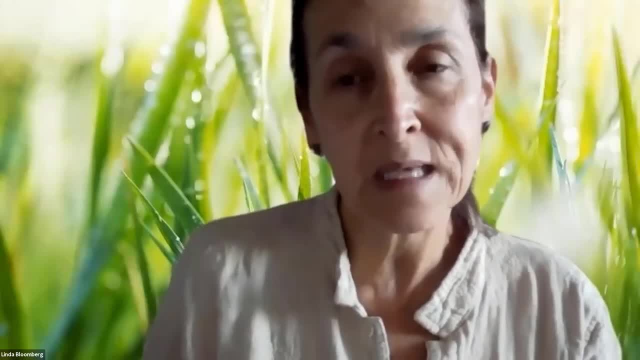 under the defense calendar, So everybody is always welcome to attend any defenses that you wish, And it's a great learning experience. But if you're interested in Janelle's research specifically, which I'm sure many people are right now after hearing this presentation, 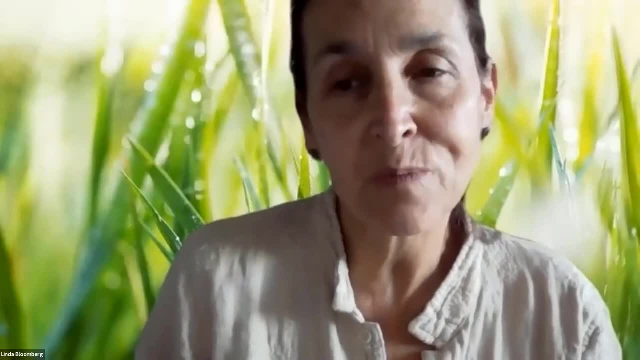 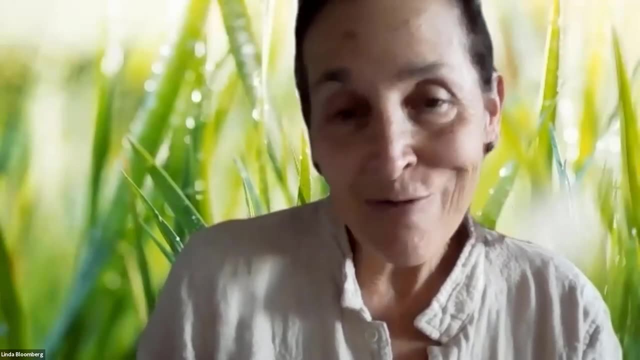 then please do come along and share Janelle's very special day at her defense, and I will let you know. So, Janelle, it looks like everybody thought this was excellent And I really thank you. I thank our participants, And if there are no more questions, we can end. 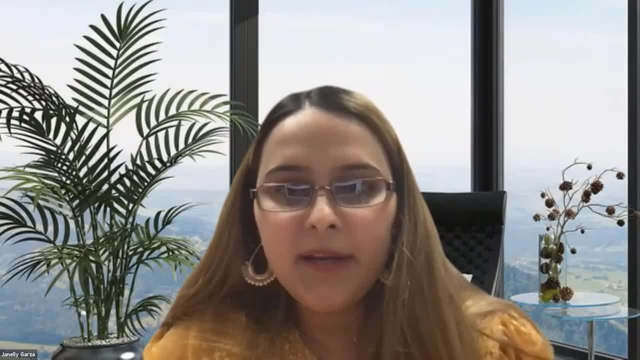 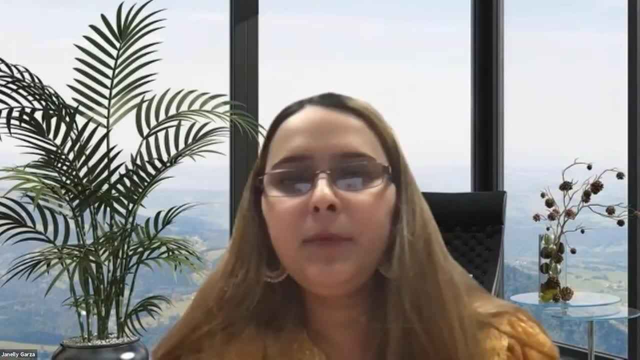 Yes, I want to thank everybody And I'm just going to post my email on chat just in case anybody wants to. If you would like to contact me at any point, you all can send me an email. I'll be more than.